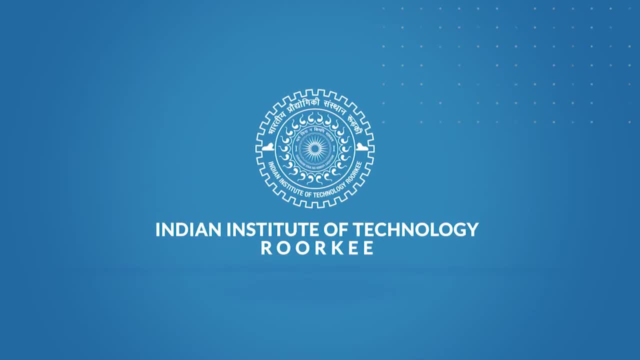 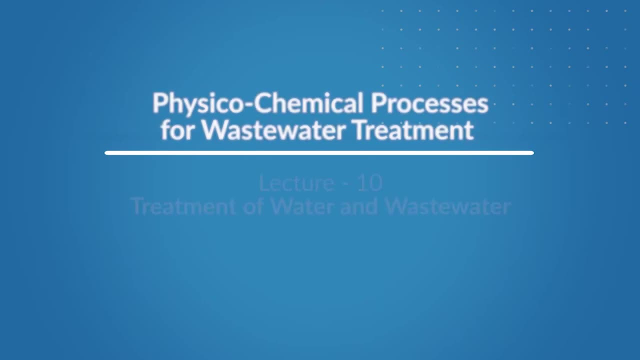 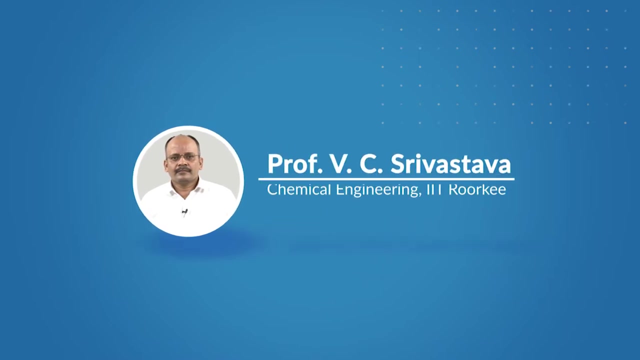 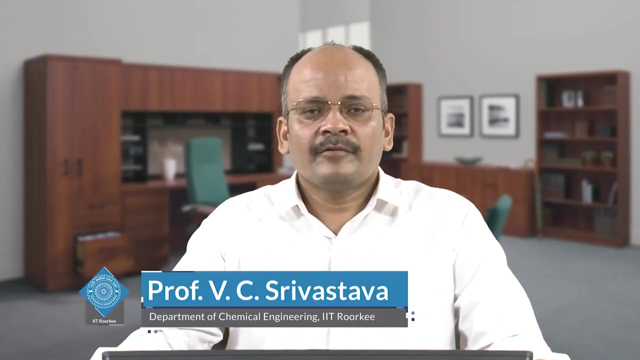 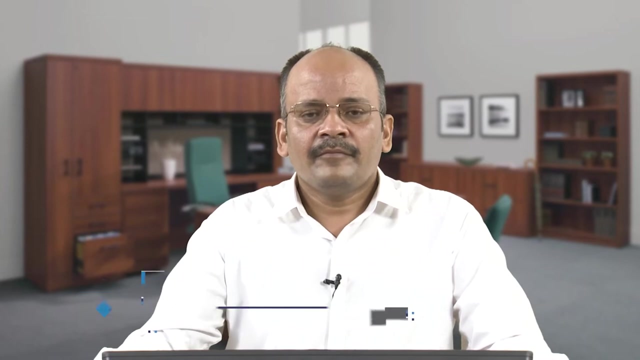 Good day everyone and welcome to this course on Physicochemical Treatment of Wastewater. So in the previous lectures we studied regarding the various methods which are there for quantifying or qualitatively analyzing different types of wastewaters And we understood various 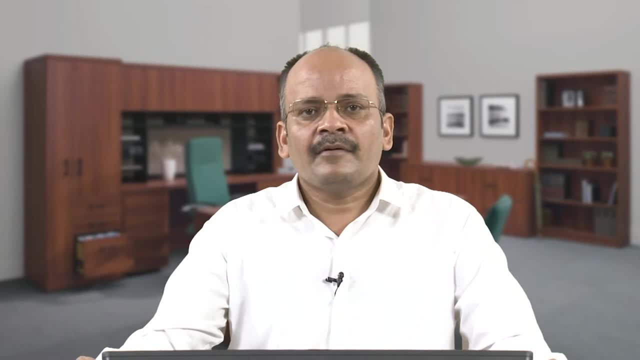 physicochemical parameters, as well as bacteriological and biochemical parameters, which are essential to understand the different types of waste. So we studied about different other components which are present in the water and how these parameters affect the treatment process, how they affect the toxicity and other parameters. 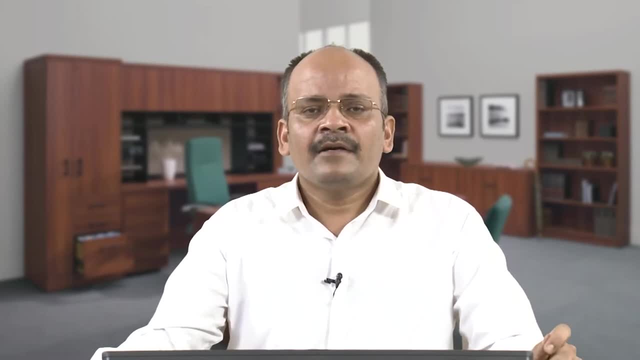 which are essential and based upon which we can decide that what type of treatment strategy we are going to adopt. So all the previous lectures were based upon those methods, understanding those methods and also trying to know what are the standards, what are the acts and regulations. 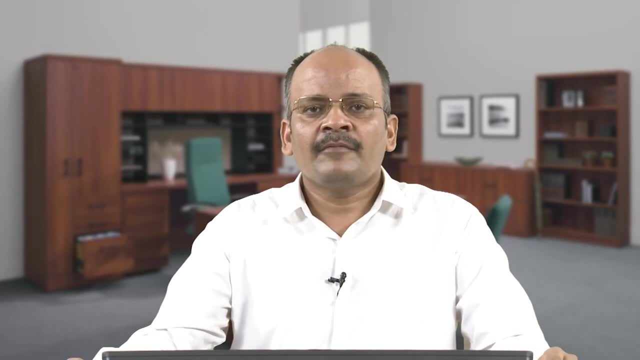 etcetera, with respect to treatment of water and wastewater, And also analyzing the various sophisticated instruments which can be used for understanding the chemical composition and other characteristics of the water before treatment as well as after treatment, So that we can analyze- analyze the efficiency and the mechanism by which the removal is happening inside any 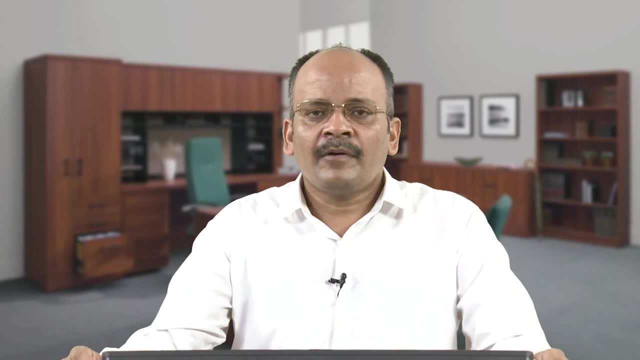 treatment plant or treatment unit. So from today's lecture onwards, we are going to start that the understanding the treatment methodologies which are being adopted for treatment of water as well as wastewater. So these, from today onwards, we will try to learn each of the units in detail. some 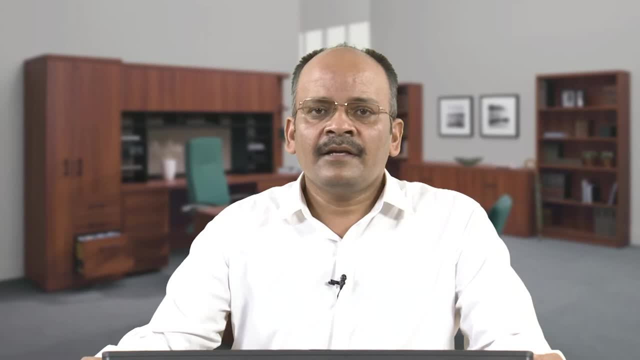 design aspects, will be understanding and then also doing some numericals and other things so that we can better understand all the mechanism as well as the design aspect of the units, Now why we require water to be treated. So this is illustrated in this slide. 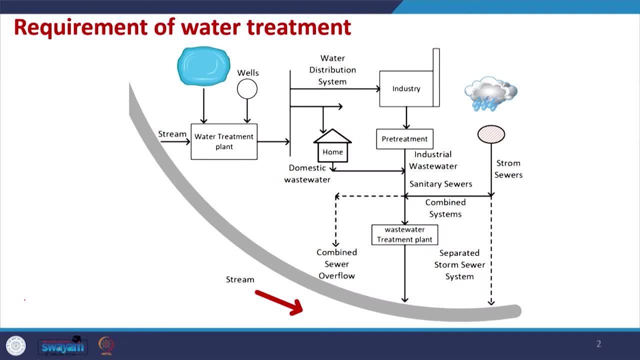 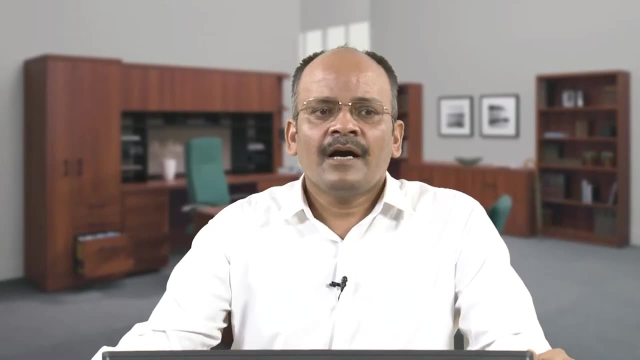 So for water. water is used in our day-to-day life, and in our day to day life what we see is that we use water for drinking, we use water for bathing, as well as for various other needs which are there inside our household. 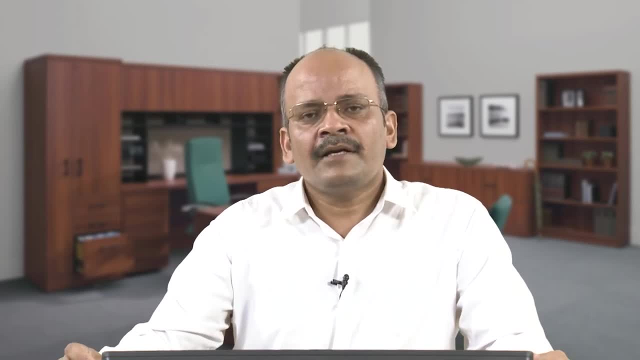 In addition to that, we see that water is also used in the industry for various uses, and from there the wastewater is discharged. Similarly, after uses in our home, lot of water is discharged and that has to be further treated or discharged into any aquatic stream or otherwise. 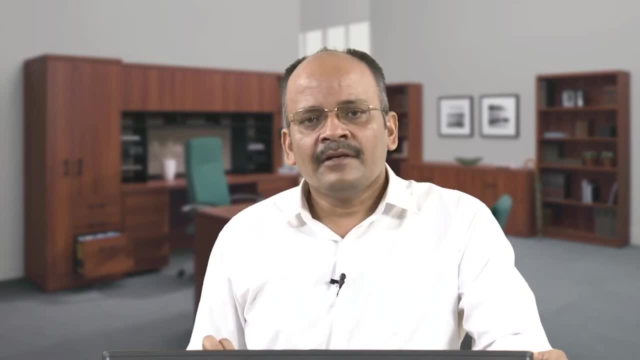 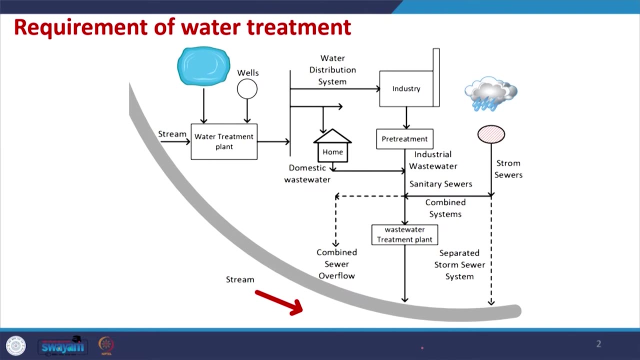 So there are essentially, if you see, most of our cities are located in those areas where water availability is very high, And so that is why, in the earlier prehistoric ages, and after that also, most of the well-developed cities are always on the banks of some river, so that the 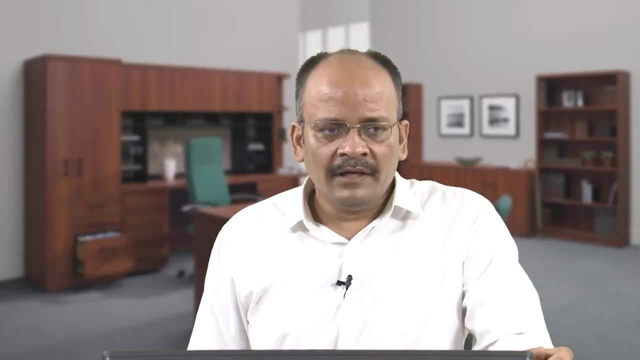 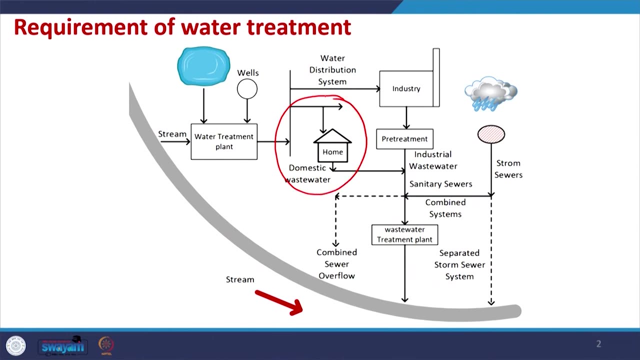 water requirement is always met, So in any city or any residential colony, if we can consider like this. So here the water required can be met from two sources: 1. Water, 2. Water, 3. Water, 4. Water. 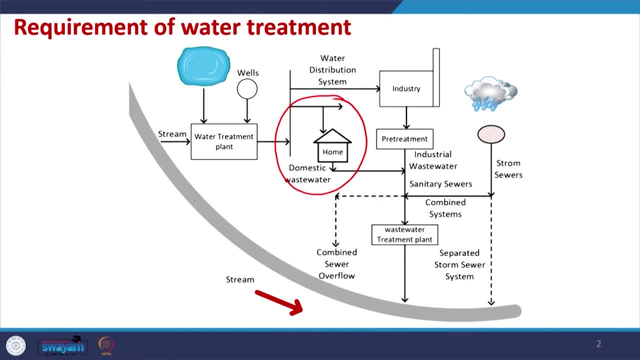 5. Water, 6. Water, 7. Water. The source is like any of the stream, like river which is flowing, and also there may be lakes and reservoirs from which the water can be taken, and similarly, from wells also water can be taken. Now, if the quantity of water which is being taken from river lake, 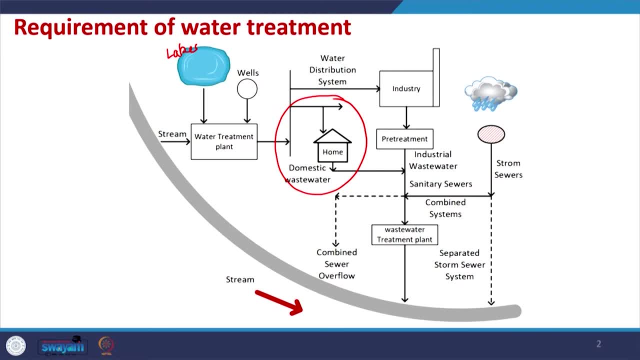 reservoir or wells. it is not good enough that we can directly use the water, So that water has to be treated. So we have water treatment plants which treat the water from any aqueous system for further use in homes. Similarly, there is lot of water requirement in the industries. 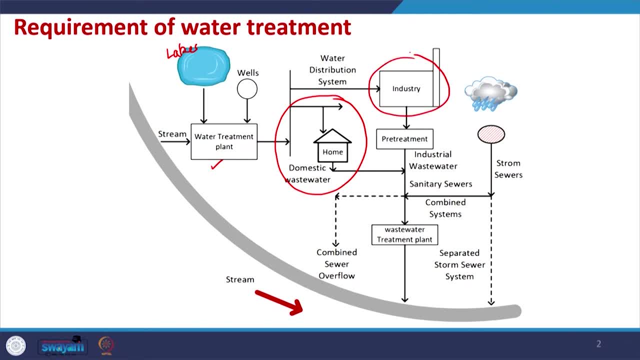 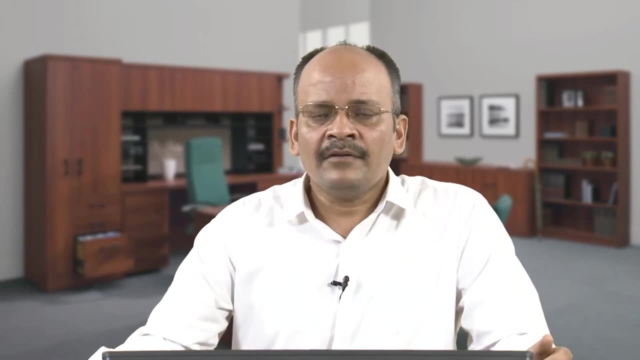 also. So there may be an industrial cluster or an individual industry may be located in any city or outside that city, So for that also water is required. Now that industry may also take water from lake or reservoir stream or wells, It may take ground water, certainly via 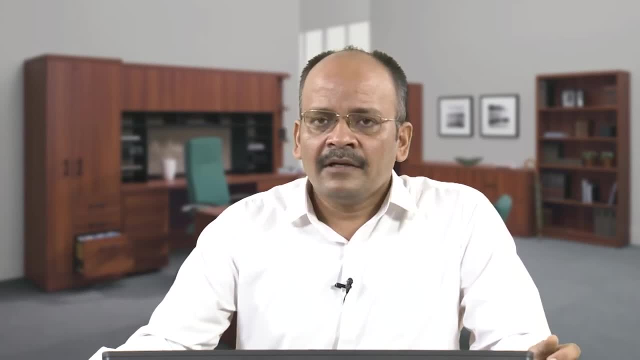 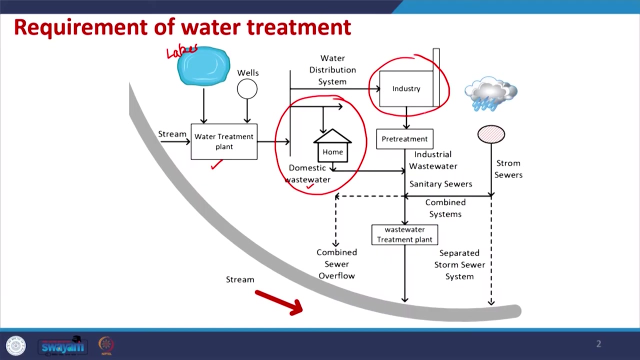 tube wells, etc. So that water is further used in the industry and after uses they try to recycle, maximize the use of water. Still, some amount of water has to be discharged. So we have domestic wastewater Which is generated, and then there is a industrial wastewater which is generated. Now, both of these. 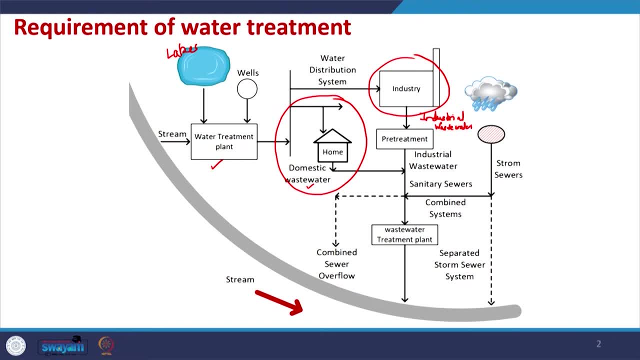 wastewaters have different characteristics and they require treatment before they can be discharged into any aquatic stream or use for any other purposes, also like agriculture, Now, many industries. actually, what they do is that they have to treat that wastewater up to a certain level and then they have to take it to the next level. So they have to take it to the next level. 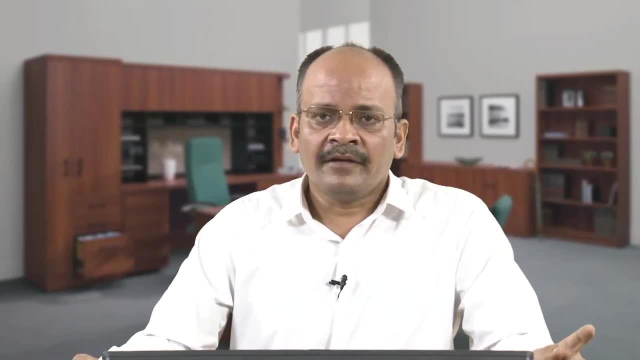 So they have to take it to the next level, and then they have to take it to the next level. So they have to take it to the next level, So they have to take it to the next level, So the limits of which are prescribed in the MNAS standards, and they have to treat the water. 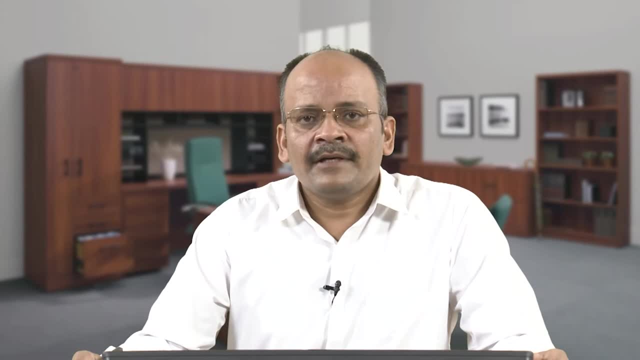 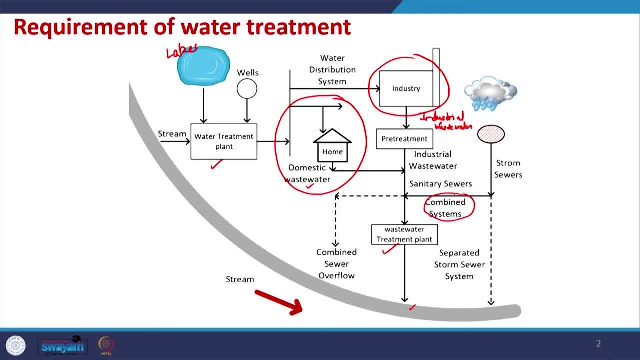 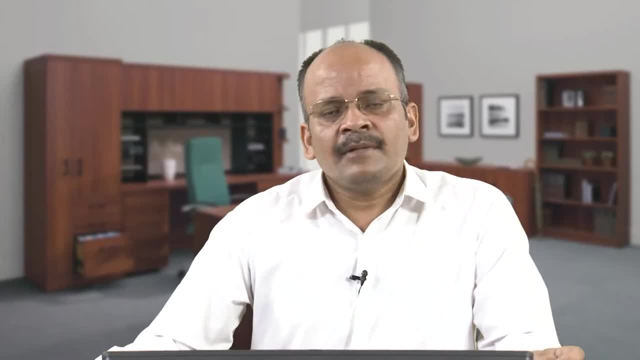 which monitor all these aspects. Many times, the standards are met by the CPCB or State Pollution Control Boards. Actually, it is possible that there may be a biodegradable treatment for industries and for entire엔 the year. Next the international08. Next, the international08. 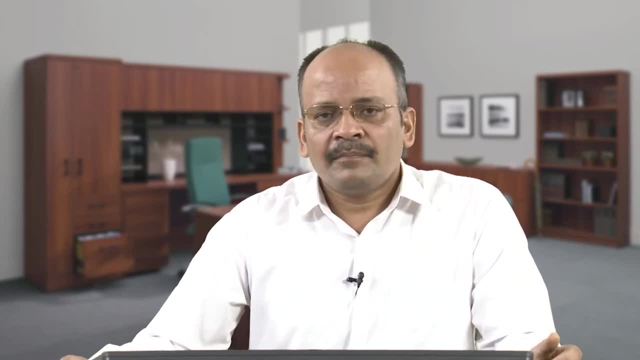 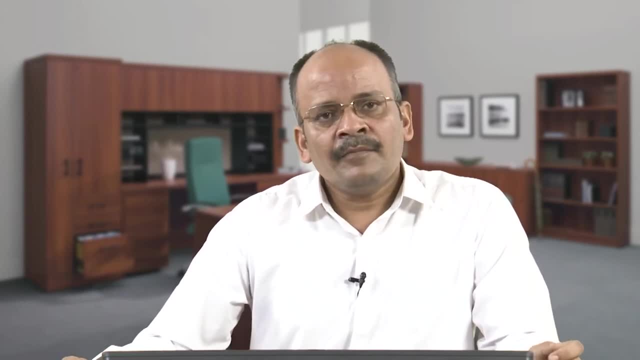 also. So that is why, overall, we require water treatment before uses and after uses also: Before uses for maybe making it potable for drinking or making it good enough for use in the industry, and after treatment so that we can discharge the water in any system or use it for any other. 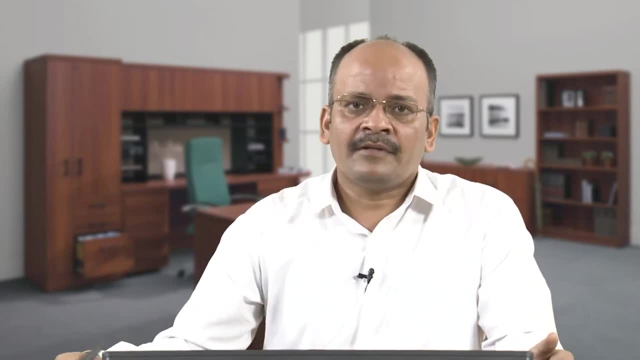 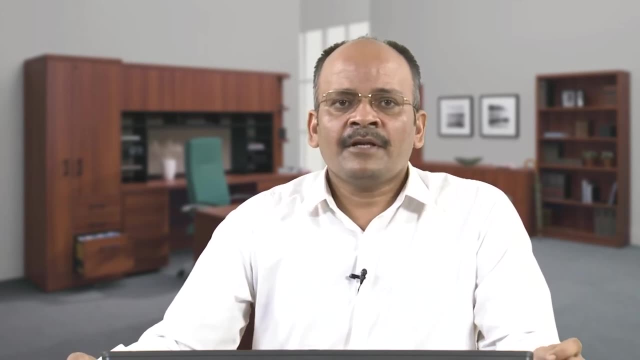 application. Now there are certain terminologies which are there in the water treatment systems. So those terminologies we should understand and what are the places where water treatment or wastewater treatment systems are used. we should also differentiate between them. Now, water treatment for use for further use in the. 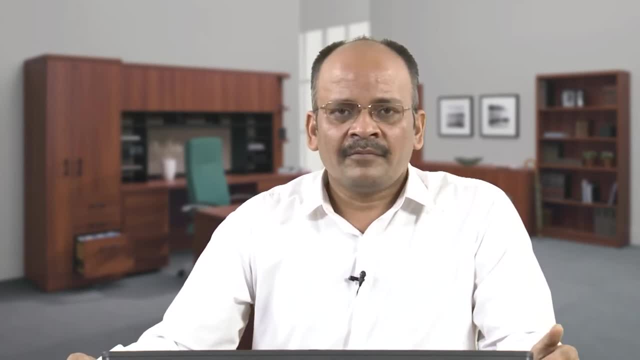 domicile. In domestic cases we have two types of generally treatment systems. One is like point of use treatment system, where we have in our own residences, small treatment units are installed which contain some of the basic units, like adsorption, RO and, depending upon UV, may be. 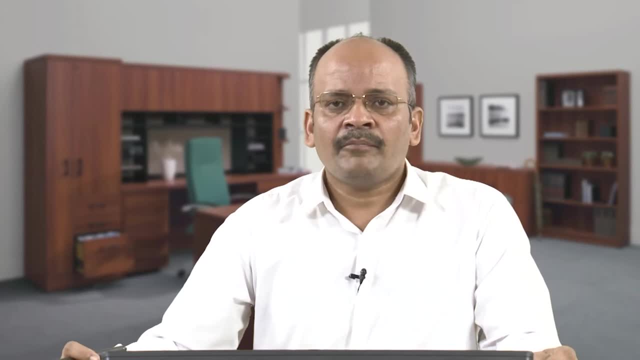 there some filtration systems, So those are there, So those are point of use. treatment system Also, there is a possibility that community treatment may be there. That means we have a bigger plant which actually treats the water which is being taken from a stream also or from the groundwater. So groundwater is commonly 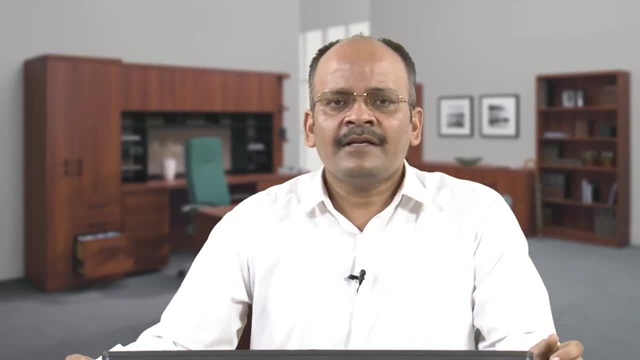 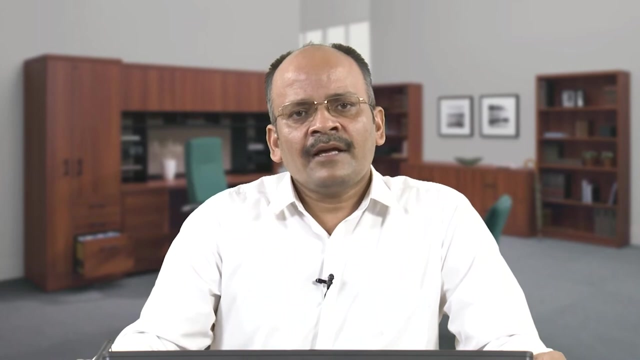 taken in most of the small cities. and then it is further. some treatment. basic treatment is done in the, either the water storage tank or before that. So this way we treat the, So that may be considered as the community treatment Now after uses of the water in our residences. 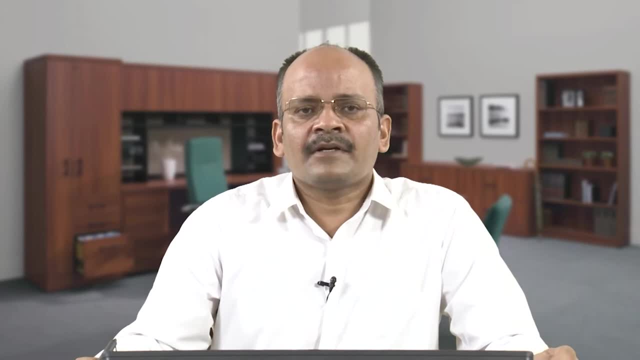 what we discharge is generally terms as municipal wastewater, because this is discharge in the from various municipal bodies, and all those water is further collected. We have a sewerage system for collection of these wastewater and then it is taken to a place where the treatment is them done. 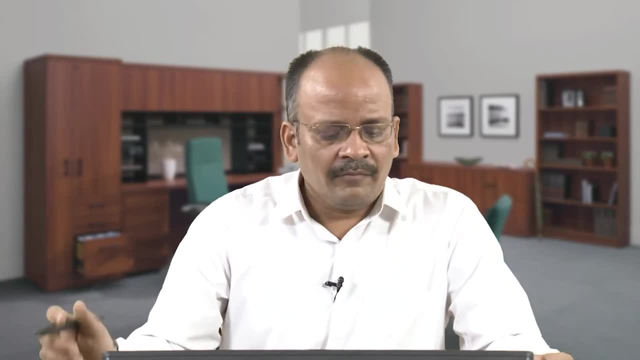 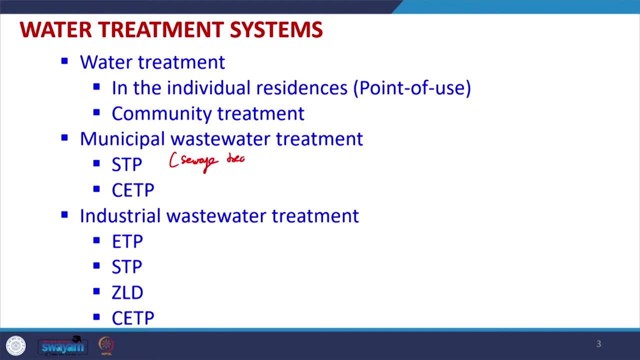 Now there are two terms which are very common. One is called STP, So STP is like it is, referred to as sewage treatment plant. So these units are there. These units are generally smaller as compared to other types of units, like CETP, which is 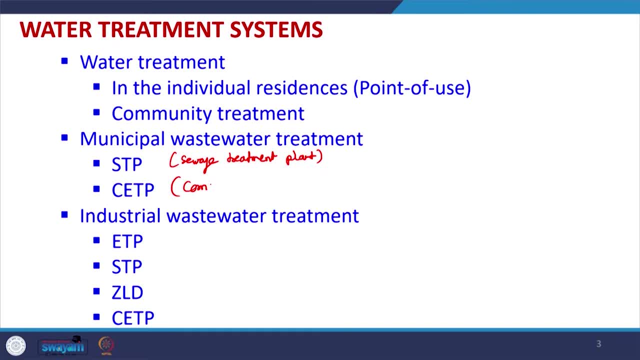 called as common effluent treatment plant, So sometimes this in place of STP- we have common effluent plants where the water from industry as well as municipal wastewaters are combined together and they are treated further. So there is a possibility of common effluent treatment plant also being used for treatment. 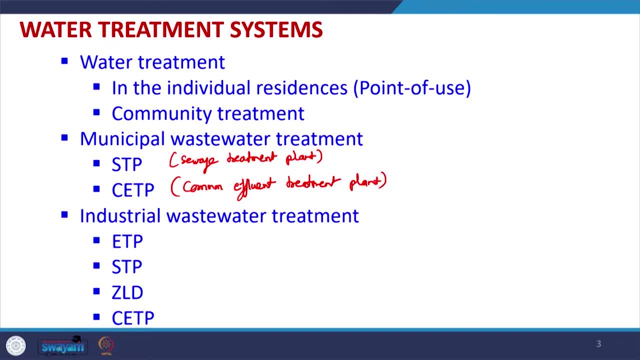 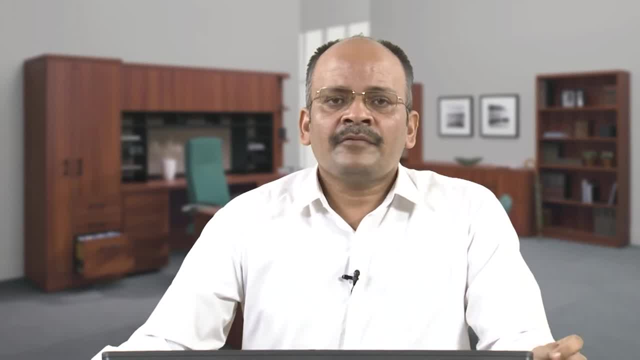 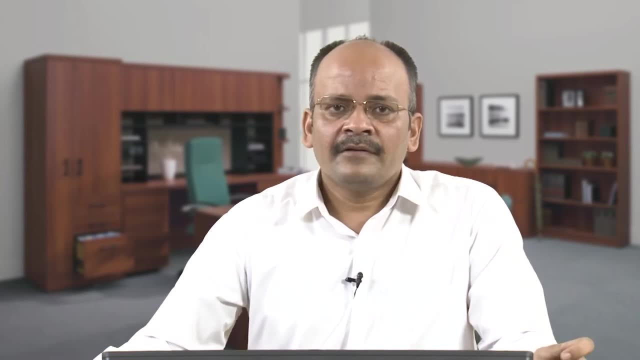 of municipal wastewater, but generally it is lesser common. So this is there. Now there is. another possibility is that since water is being used in the industry, So lot of industrial wastewater, which has characteristics much difference than the municipal wastewater, may have, has to be treated. 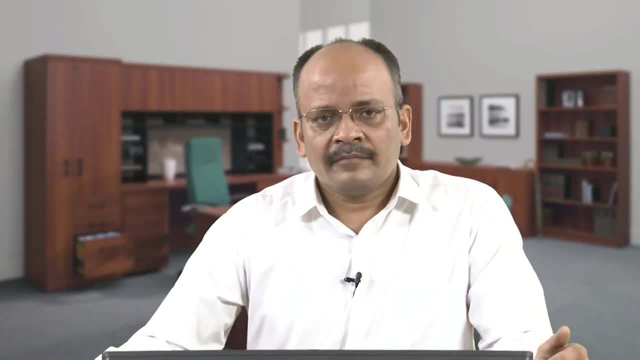 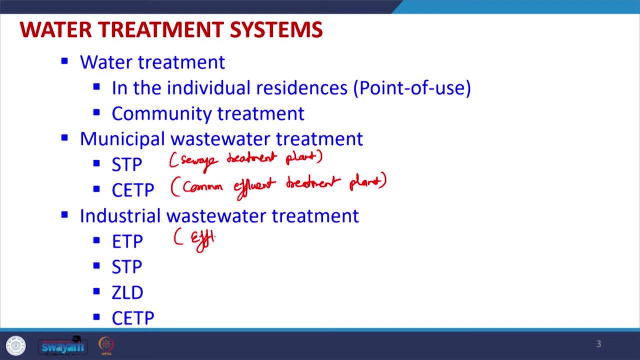 Now this wastewater treatment plants are named. a number of abbreviations are used commonly during the treatment And those are called like ETP. ETP means effluent treatment plant, So that means generally we are here referring to the wastewater which is getting discharged. 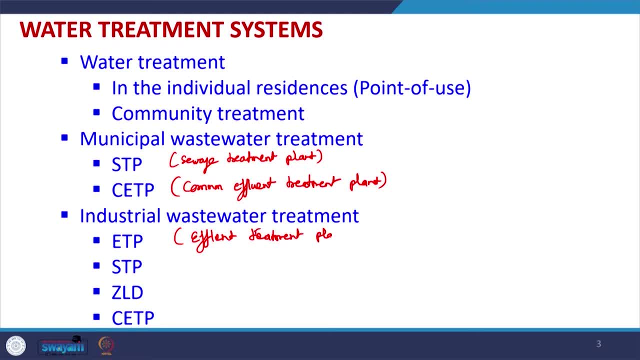 from the industries and it is being treated in a treatment system which will generally be at least three stages. So effluent treatment plant must be there in any industrial Waste industry where some industry wastewater is coming out. Now many a times we may feel that any industry which is not generating any pollutant may. 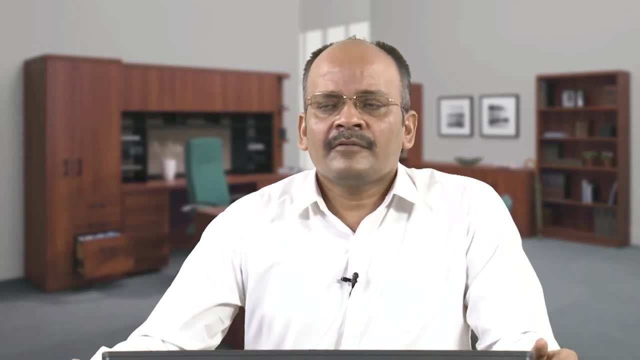 require no treatment of wastewater. So like any electronic industry, suppose it is there. So for electronic industry we will consider that in the electronic assembly unit there is no use of water, So that means they are not discharging any industrial waste. 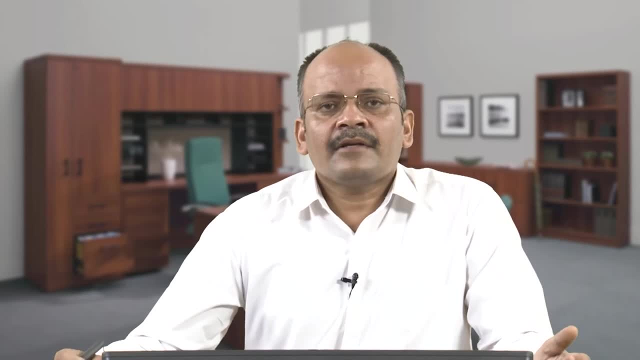 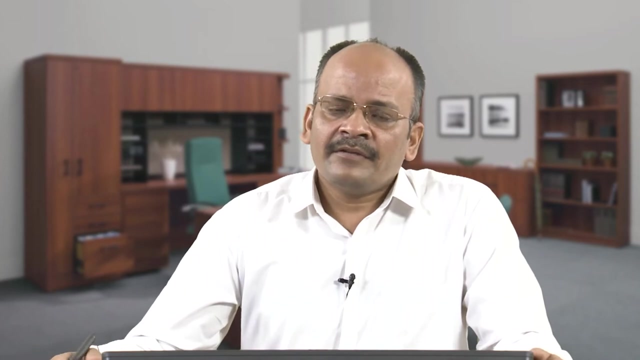 So there is no treatment required? Yes, logically it seems so. but any electronic industry or in any other industry where the water is not being used, but still there are number of persons working in that industry And there they are using the water they are and further discharging the water in the laboratories. 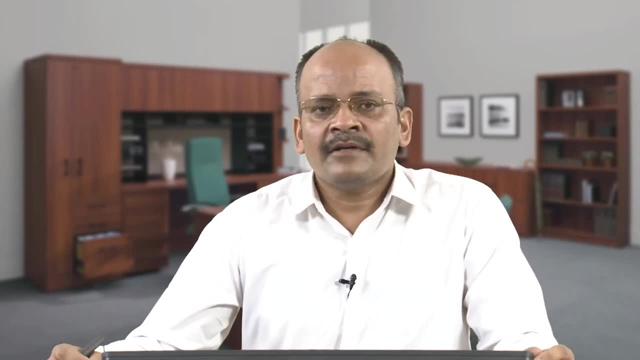 also. So that means they have lot of urethane. So that means they have lot of urethane. They are using the urination. all the people are urinating as well and they may be using. they may be generating some other types of wastewater also and sewage. 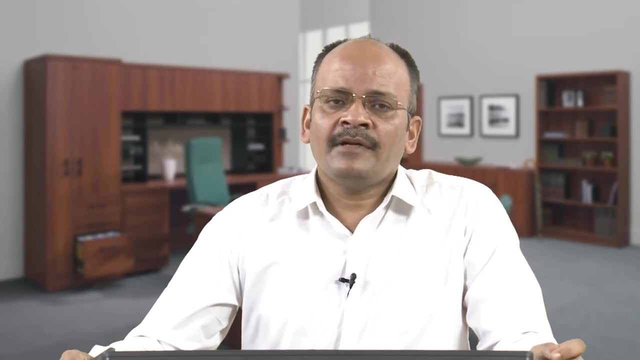 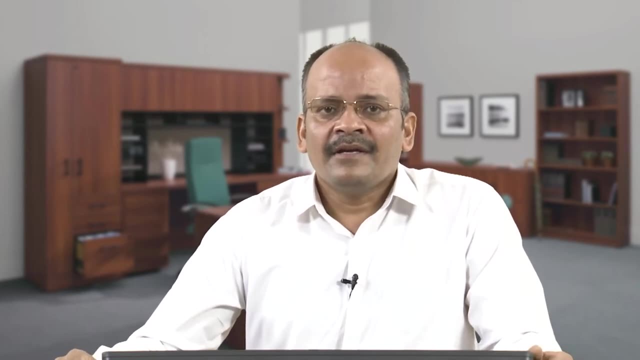 So that means any industry which is having number of persons working beyond a certain limit, they have to install a STP which is like a sewage treatment plant, So they cannot discharge the water as such. Still they have to install a STP. 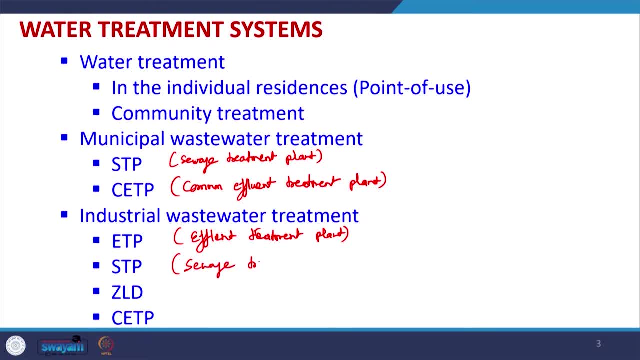 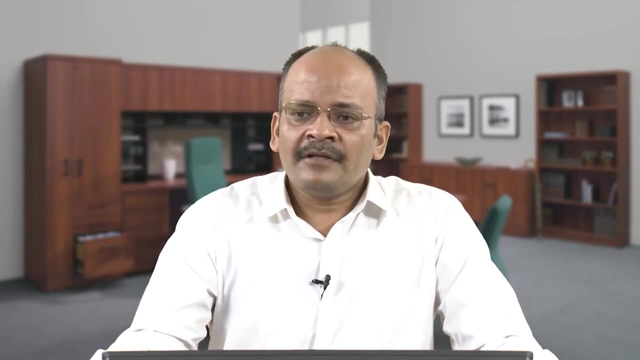 Okay, seawaste treatment plant in those industrial units also where there is, as such, no generation of industrial wastewater, So these units also need to still need to install the seawaste treatment plant. In fact, nowadays there are guidelines that hotels, all those places where 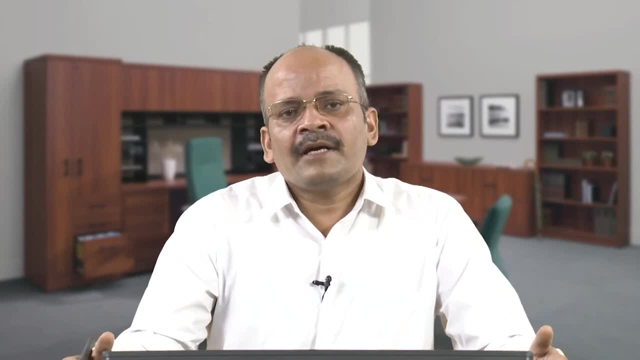 there are persons beyond a certain limit at a time, Then also they have to install a simple basic unit for treatment of water which is getting generated in that place, and then only they can actually do business and run that particular thing for any business, etc. So this is very, very essential and this is true for hotels, restaurants and many other. 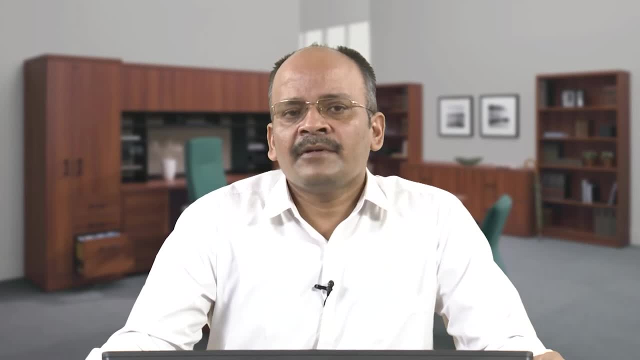 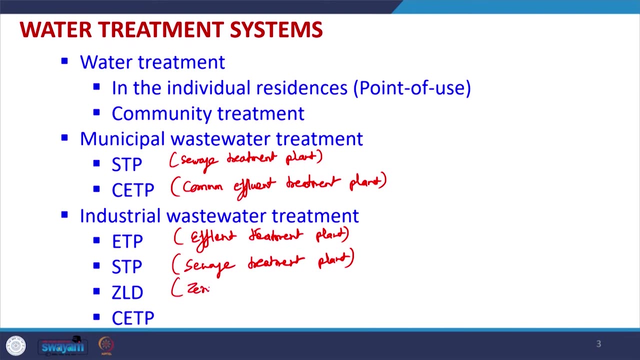 places also. So these treatment plants have to be installed. Then there is a one very common terminology which is called as zero liquid discharge. So zero liquid discharge means there are certain guidelines for many industrial units which actually generate wastewaters which are highly toxic and they have lot of pollution load. So that means the amount of pollution. 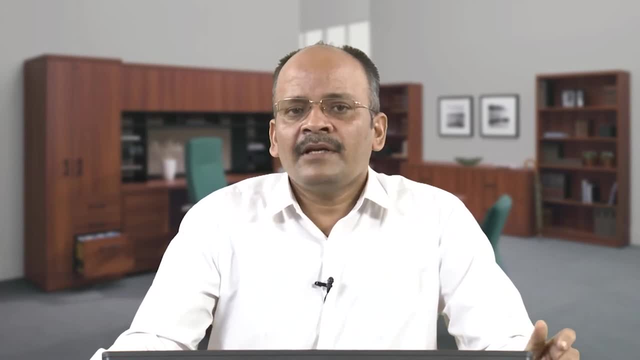 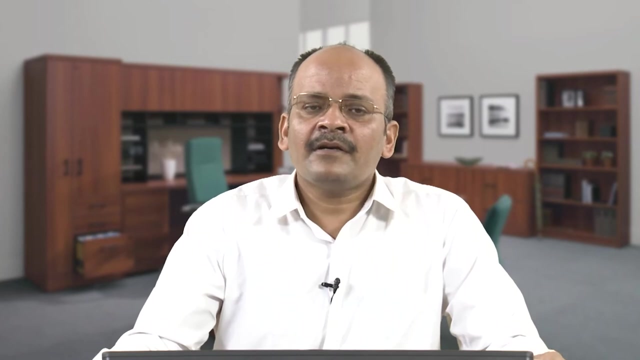 present per meter cube of the water is very, very high, And for them that- not only the treatment- is very, very essential. In fact, they are told that they cannot discharge any water out of their premises, So that means they have to first treat the water, reuse the maximum amount of water and somehow try to see that. 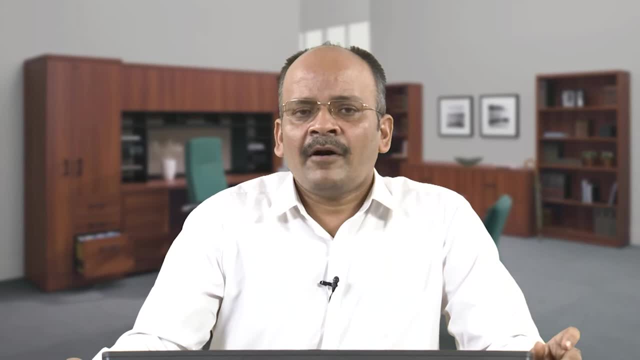 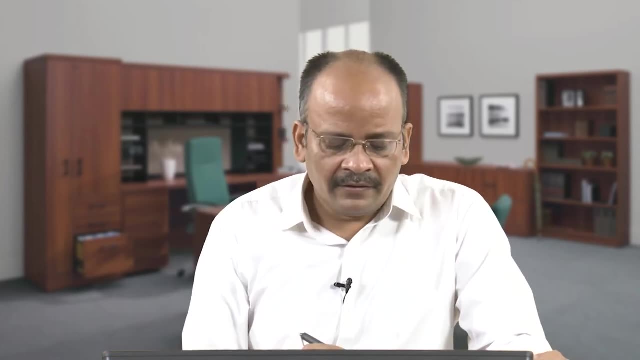 if any water is still remaining, generally they evaporate that water. So they cannot discharge any water out of their premises and that is why they. this is a very important thing. There is another system is called zero liquid discharge. So ZLD So many times for these. 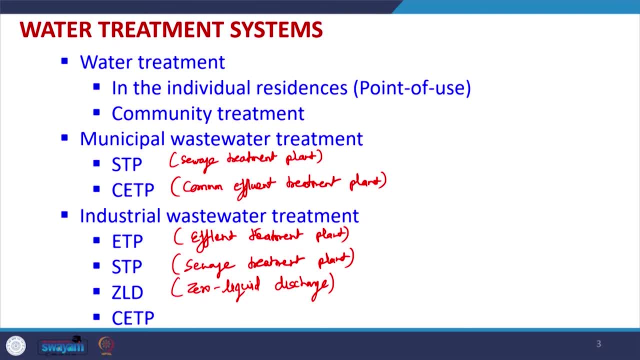 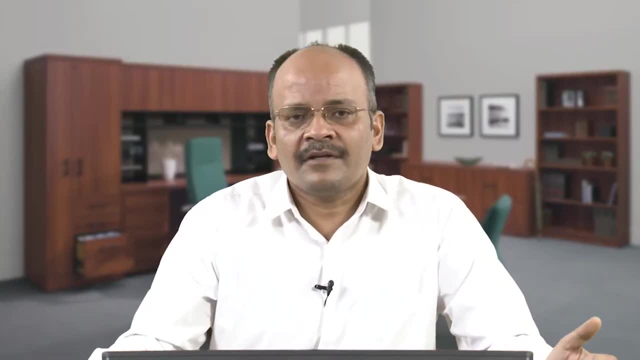 industries. in place of taking the name ETP, they will take the name ZLD has been installed, So that means they have an ETP also and some evaporation- that type of system where they are evaporating the water may be generating steam which is further being used in the process. 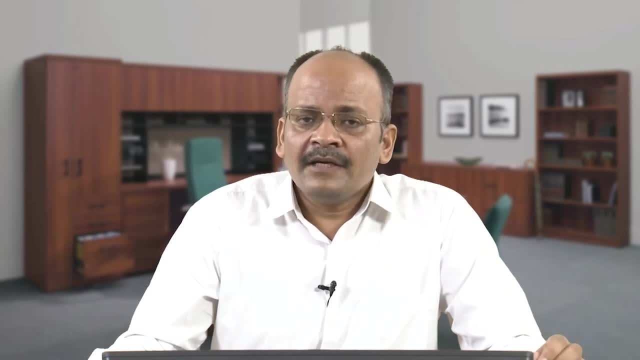 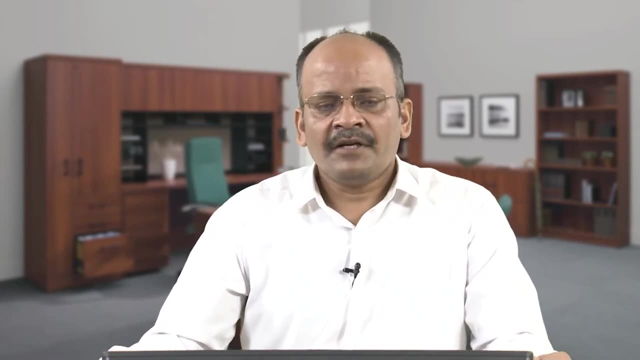 But still they have to. they cannot discharge any water out of the premises, So this is very important. So that means they have ETP also and some other type of system where they are very essential. Then there is a common effluent treatment plant when we have a cluster of 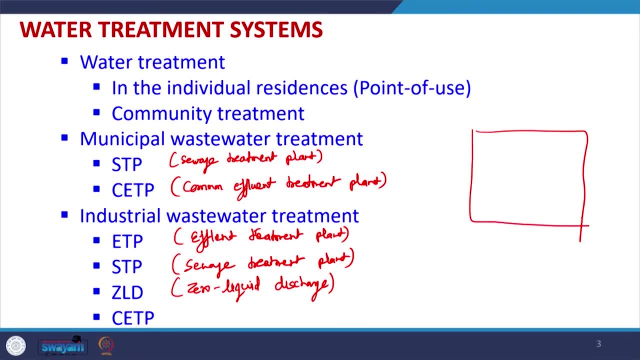 industries are there. So what they do is that, suppose this is a big cluster and they have different industrial units which are there, and so what they do is that they will discharge water. everyone will discharge water after some treatment. So what they do is that, because these industrial 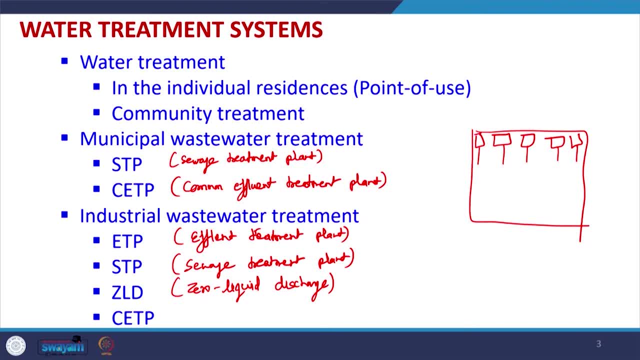 units may be entirely different from each other with respect to production, So that means the water which is getting discharged from these units may also be entirely different in terms of characteristics. So that means what they do is that they treat some amount of water in their 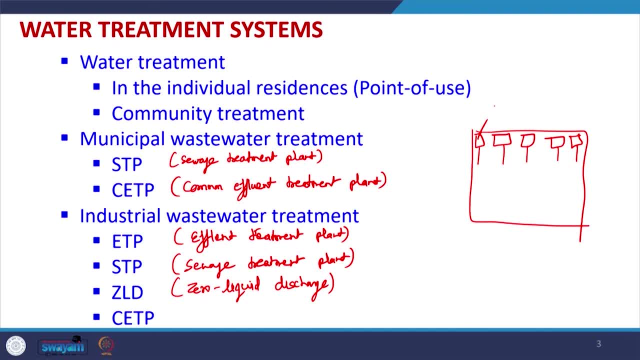 premises. So this is like: suppose this is industries- I am just putting industries 1,, 2,, 3,, 4, 5, etcetera. So that means they will be be having some primary treatment, some treatment which may not be fully treatment, but some. 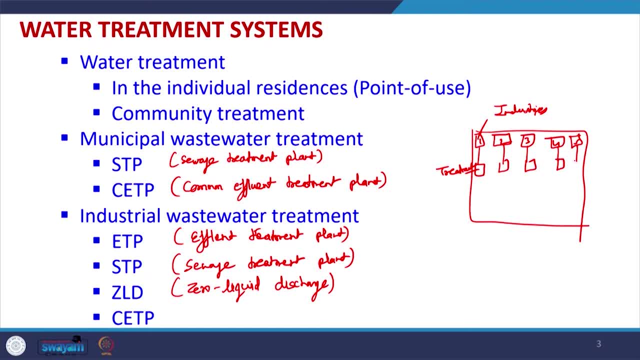 treatment may be done and after that, whatever water they discharge, that that will be taken and treated in a common effluent treatment plant. And so the bigger load is on the common effluent treatment plant and they are doing some primary treatment. after that they are discharging into this common effluent treatment plant. 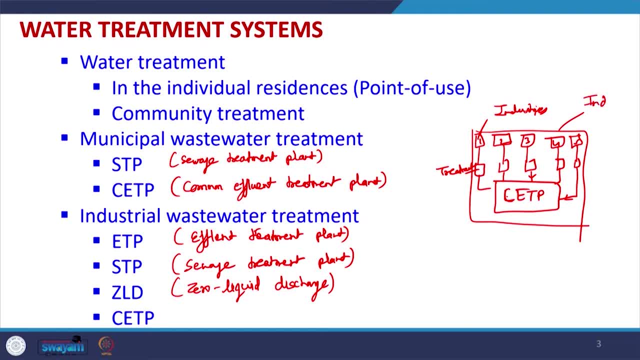 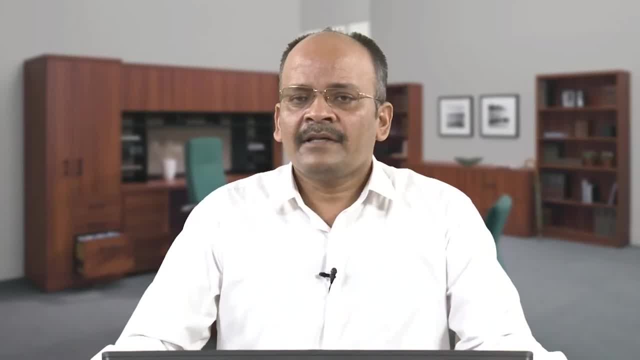 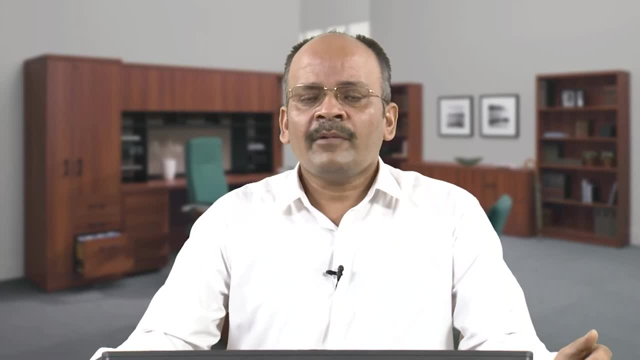 and this may be a industrial cluster may be there. So this is very, very common nowadays. so lot of industrial clusters are being developed by the state government as well as the central government, and we have lot, many industries. The good thing about this is that the industries do not have to install all the units. they 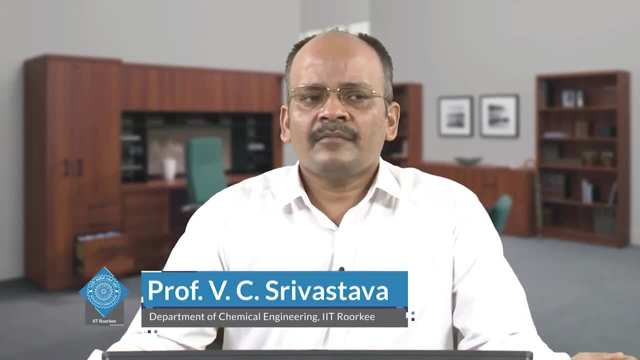 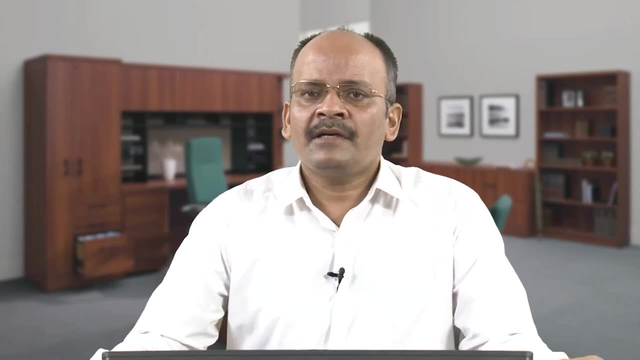 have to only do the primary treatment, and so the cost incurred is very less. certainly they have. So they may have to give some amount of money to CETP, depending upon the characteristics of water they are discharging to CETP and also amount of water. so it is, it is a mix. 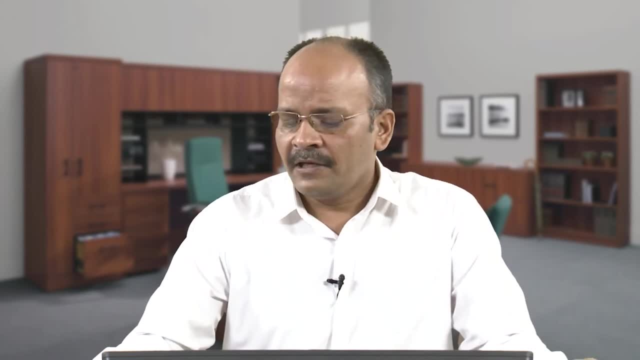 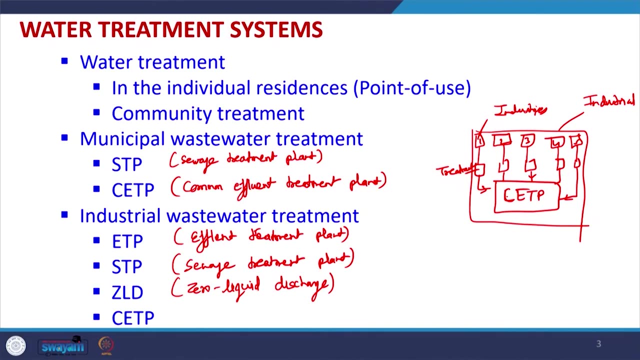 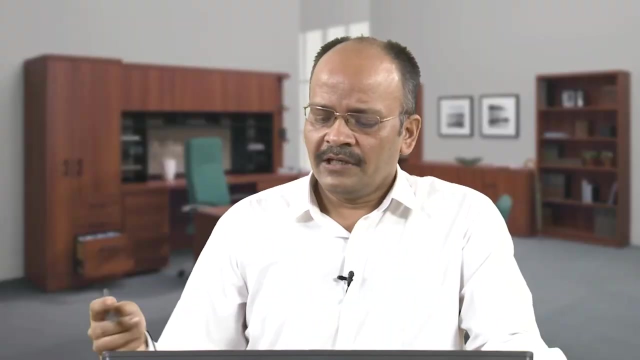 of both. So some weightage may be there and, depending upon that, monthly they may have to give some amount of money to the CETP. and CETP then treats the water, discharges or not discharging, depending upon the condition, further to any aquatic bodies or not. 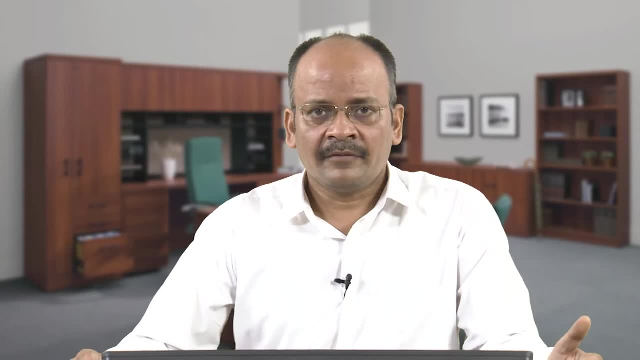 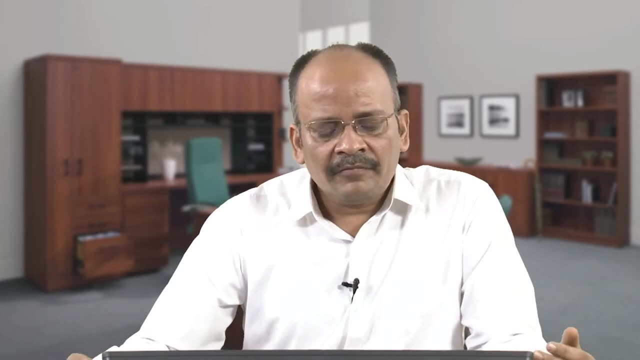 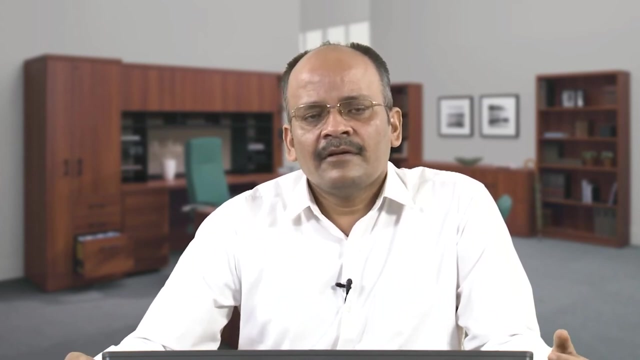 So this is the water treatment systems which are there. Now we will go further understand the water treatment systems in general. Now, wastewater treatment and disposal system generally will consist of a number of things. So first and foremost point is collecting the water- wastewater. 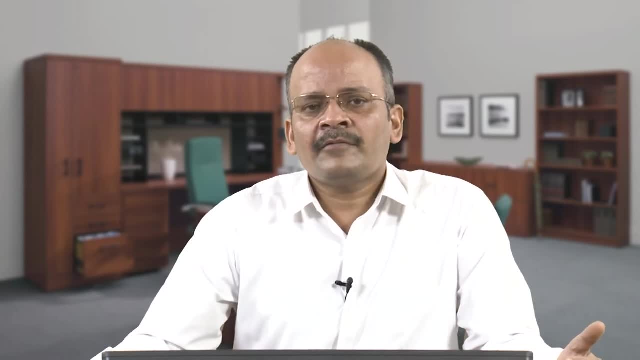 So for municipal wastewater treatment also, we have to collect. so we have a several system is there for collecting, So collecting the water similarly, for in a industrial cluster also, lot of channels, etcetera, are built for collecting the water from different industries and which is further. 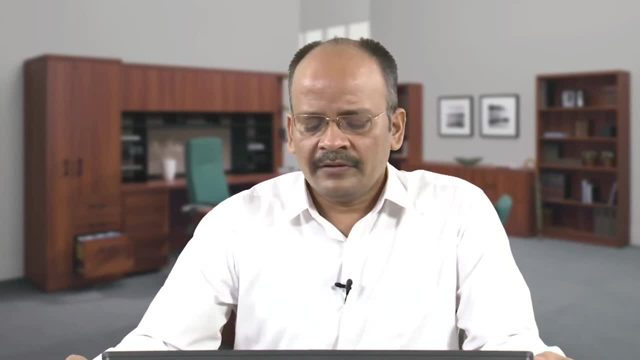 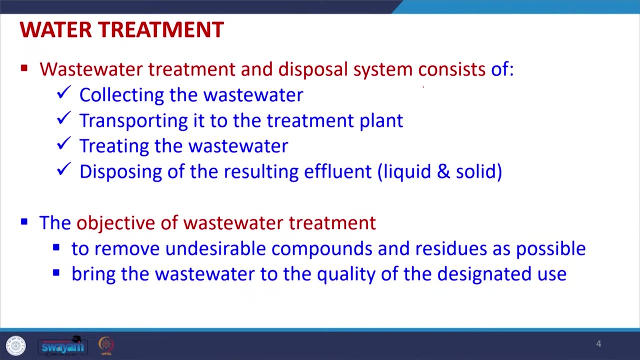 taken to a CETP for treatment. So it is there, so collecting the wastewater, then transporting it to the treatment plant. So this is essential. so in the industrial clusters which are made, it is the duty and duty of the government to make all these things, and similarly for municipal treatment. 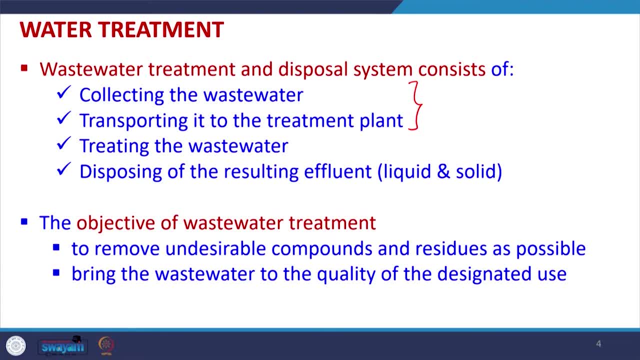 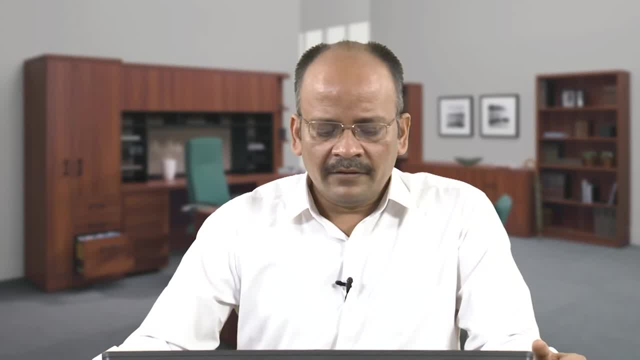 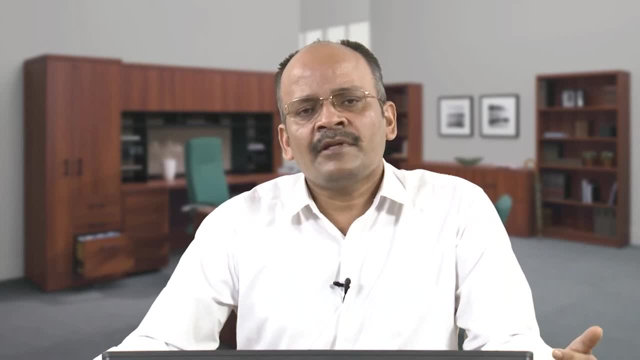 plants. also, it is essential that municipal bodies install several systems So that the water may be collected and transported to the treatment plant, Then treating the wastewater or the water in the treatment plant- So this is there- and then disposing of the resulting effluent liquid. 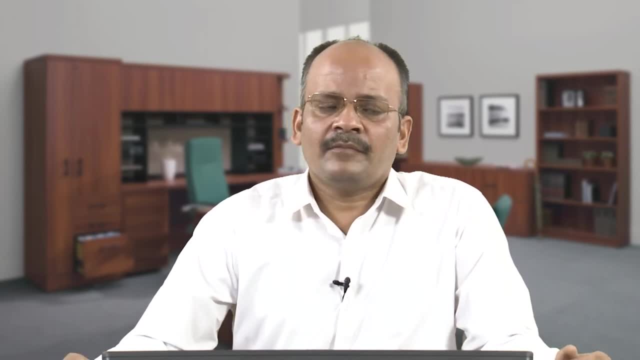 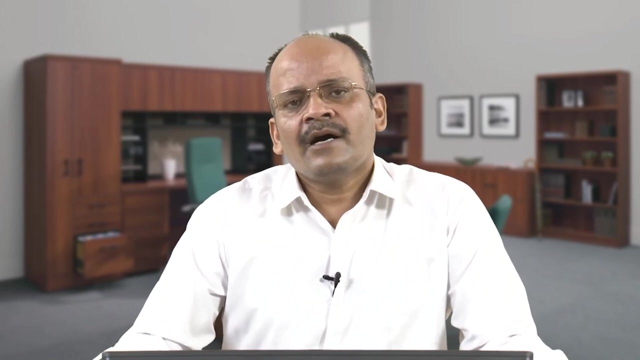 So after treatment there are two types of. One thing is the waste water. One thing is that waste water- certainly the treated effluent will be coming out, So that has to be discharge also. lot of solids, etcetera are generated And that solid etcetera also have to be treated and then discharge to the landfill or any. 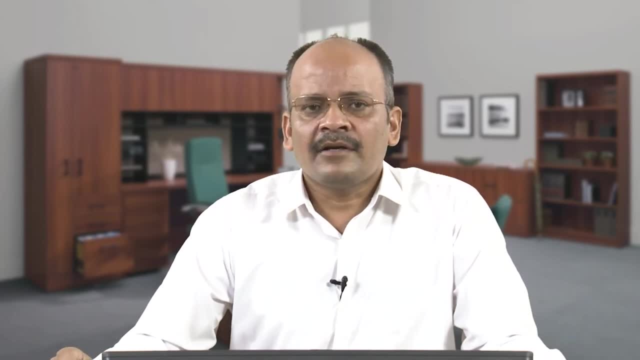 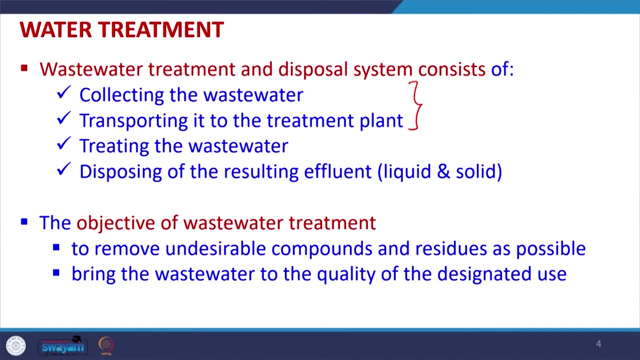 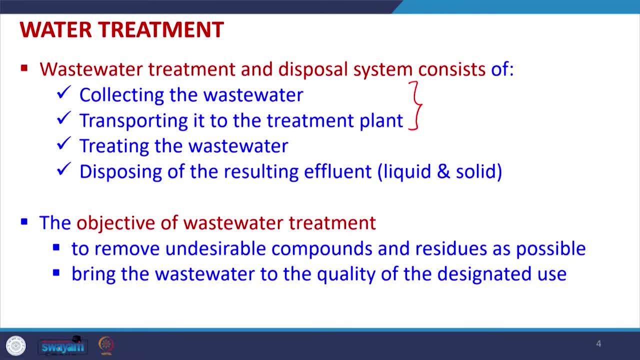 So that is the main objective of the auditoryuse welfare reform. So the main objective of this is to remove theaders, wellís and the discharge�เ� rear the sediments and several44 Forget to have that sort of water, which will also be used. 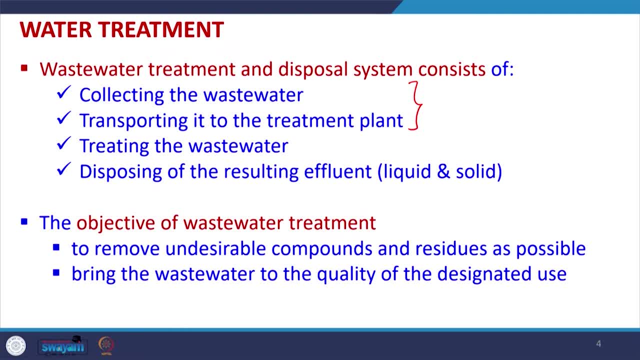 in doing the typical use of the throughput of the water treatment or an effort to avoid the damage for water using water processing actual does notמהver available compounds or residues as much as possible And to bring thewater to the quality of the designated use. 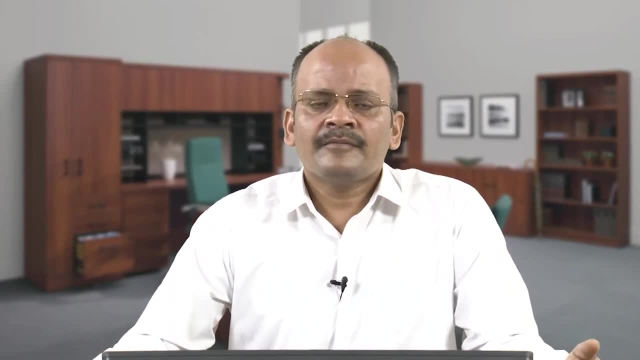 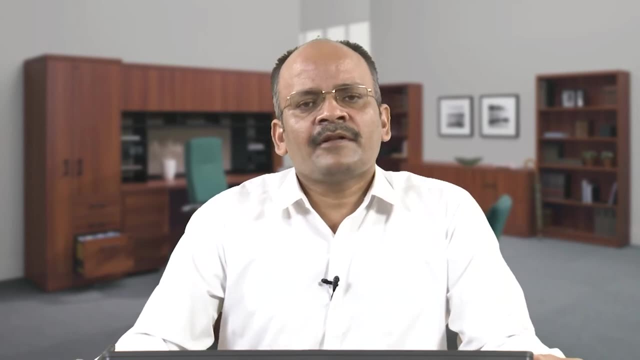 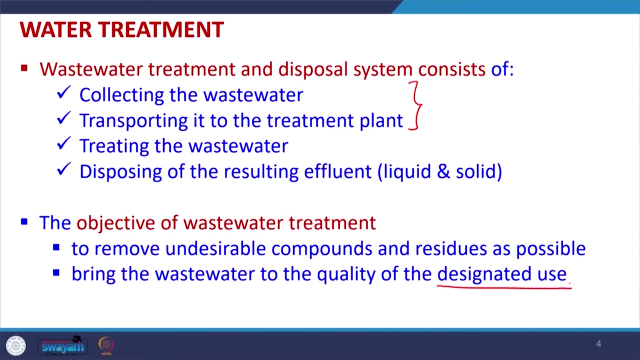 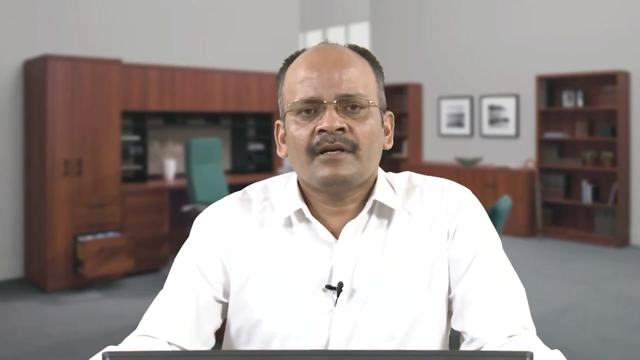 So it is possible that steam or reuse it for maybe bathing, for other purposes, for maybe as irrigation water, for further use in the agricultural fields, etcetera. So depending upon the designated use, the treatment is done further. So for some industries that different designated uses are possible, like for many industries, ZLD is compulsory. like pulp and paper, etcetera, which generate lot of highly toxic effluents and where the pollution load is high, they are not allowed to discharge any water. Similarly for some industries, since they contain some material which may be good enough. 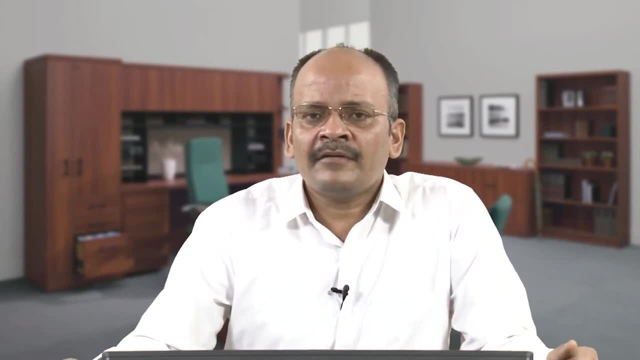 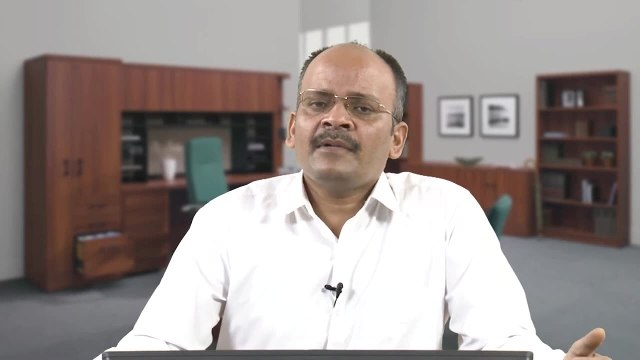 for use in the agriculture field. So, like for sugar industry, wastewater which is generated, they are allowed to treat to a certain level, So that So the water may, the treated effluent may further be used in the agricultural fields. So this is allowed for sugar industry. 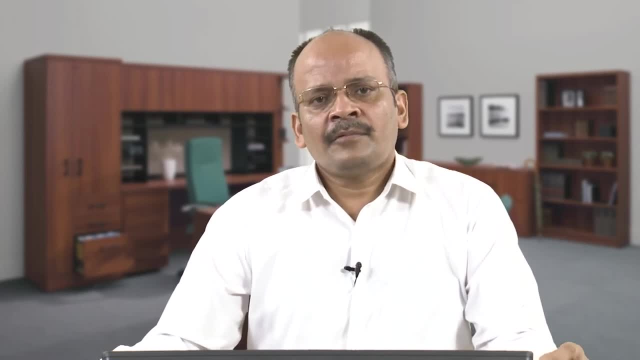 So this way we understand that the objectives of the water treatment or wastewater treatment units in different places may be entirely different. They depend upon the type of compound being present, how much amount of compound is present and also what is the designated use. So depending upon that, the objective may change and also the number of units and type. 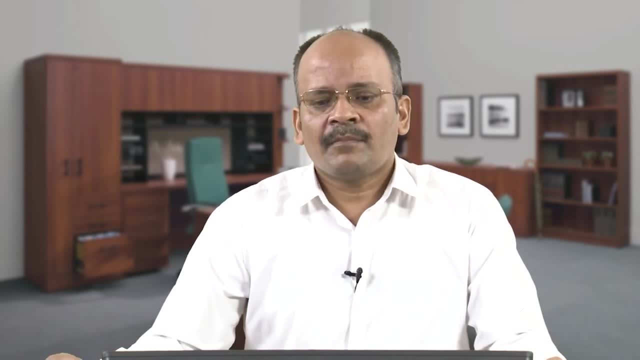 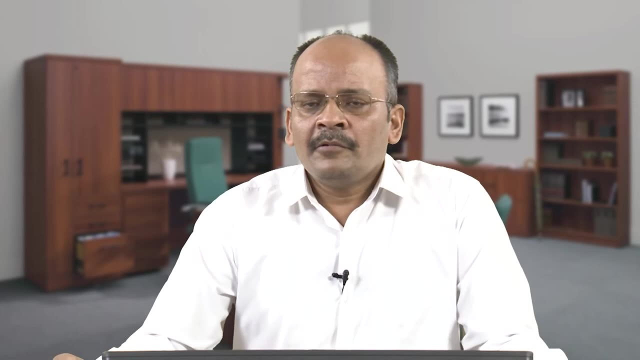 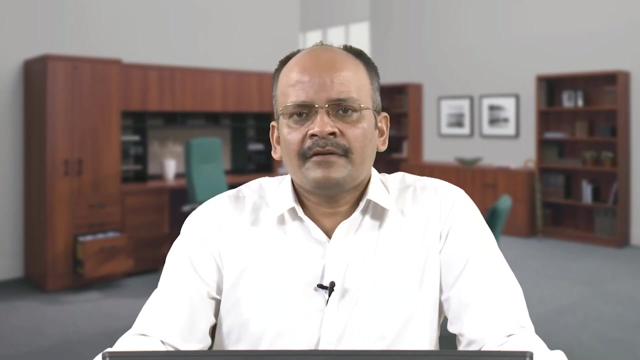 of units within a water or wastewater treatment plant may also change. Now, potable water is never produced at any wastewater treatment plant. It means that if any industrial wastewater is discharged or any municipal wastewater is discharged, Generally, So after treatment we do not use it for potable, for drinking purpose, will use it for may be. 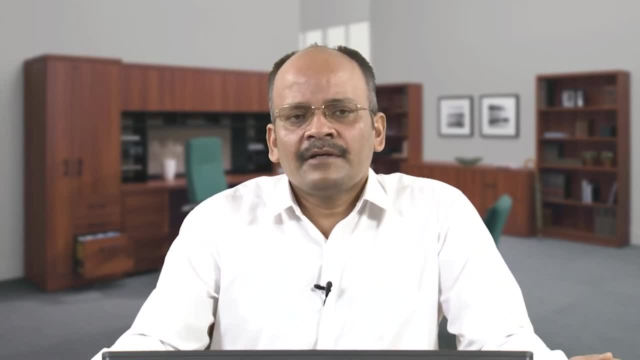 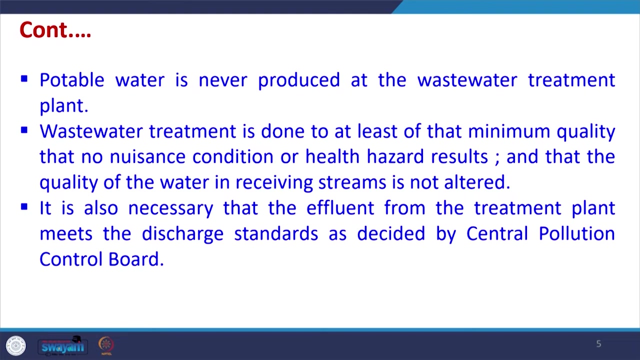 used for other purposes, but never use it for drinking purpose. Wastewater treatment is done so that we can make the water good enough so that minimum nuisance is covered or health hazards are not there when we discharge that water. So quality of 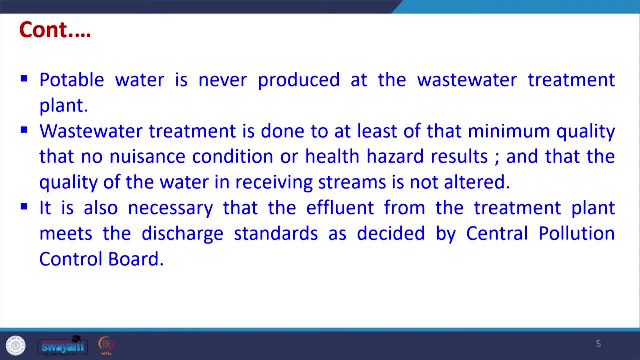 We also see that the quality of The quality of receiving stream is not altered because of the discharge of that water into that stream. So we have to make a material balance and try to see beforehand, If suppose there is a possibility that industry is there and during just besides, say, river. 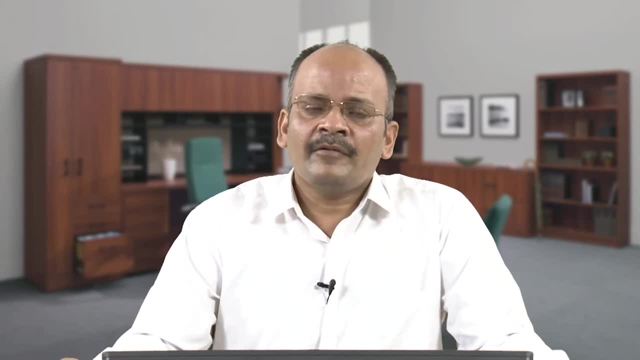 and now that river will be having very high amount of water during rainy season. So it is possible that That industry, if it discharges effluent to that river, the river quality will not be altered but will not take that condition. where the good thing may prevail, we will take that condition. 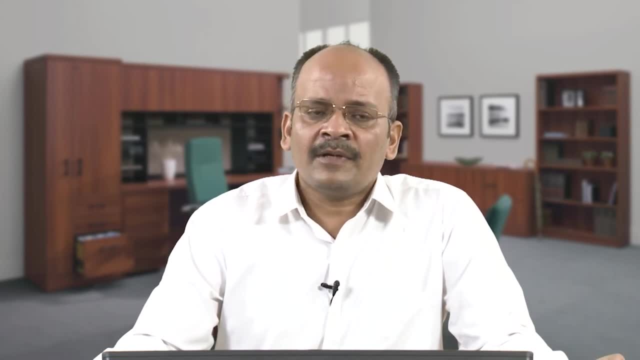 where worst condition is possible. So we will take those wastewater flow, those water flow conditions in the river. it may be in the summer season, just before starting of the rainy season, So under that condition, So under that condition amount of water flowing in the stream is very low and under. 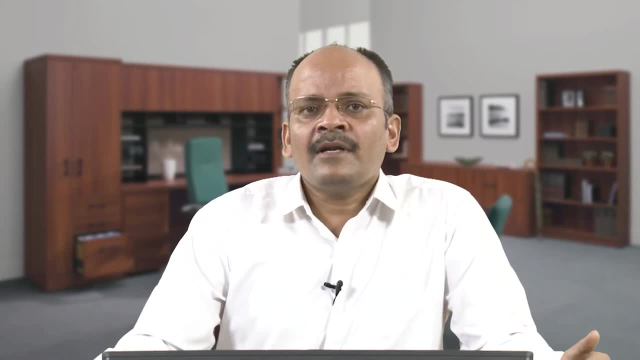 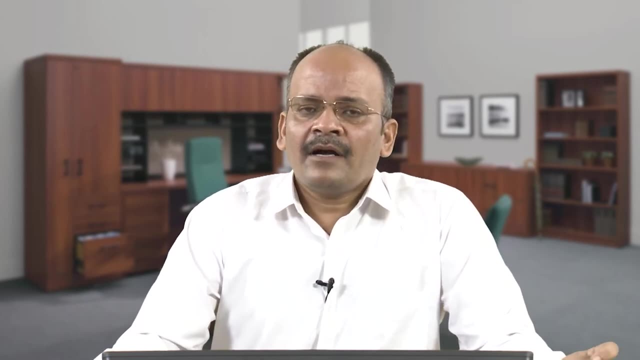 that condition. if any discharge happens, so that will alter the quality of water in the receiving stream. So that is why we will base our analysis on that condition. I will not allow that industry to discharge any effluent all throughout the season, also all throughout the year, disregarding 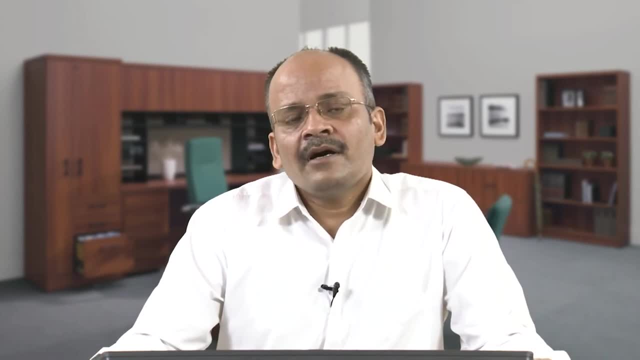 the variation in the water quality. So that is why- So that is why we will base our analysis on that condition. I will not allow that industry to discharge any effluent all throughout the year, disregarding the variation in the water quality and water quantity in the receiving stream. 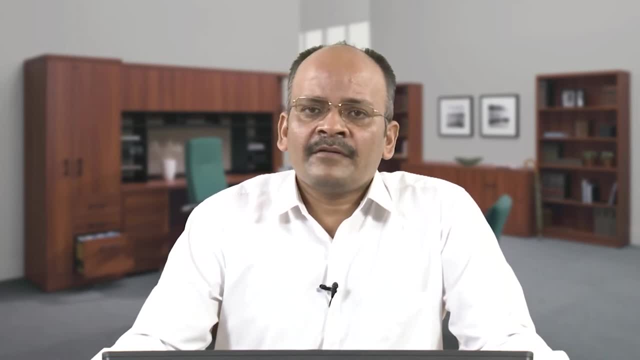 So we always should look after the worst condition and under that worst condition, whatever, whatever is the best thing that should be imposed. It is also necessary that effluent from treatment plant meets the discharge standard. So always we have to see that, depending upon the place where the treated effluent is being. 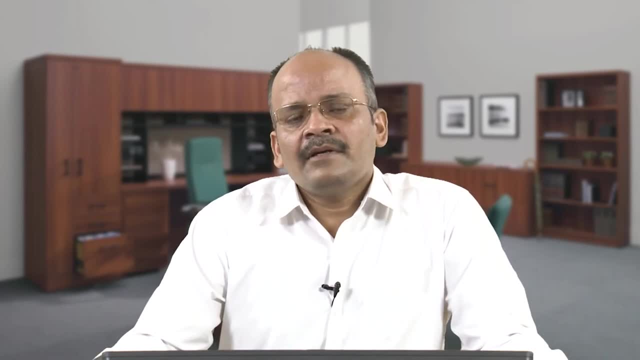 discharged. So always we have to see that, depending upon the place where the treated effluent is being discharged, So always we have to see that, depending upon the place where the treated effluent is being discharged. So we have to look after that which should be meet the criteria as set by the middance. 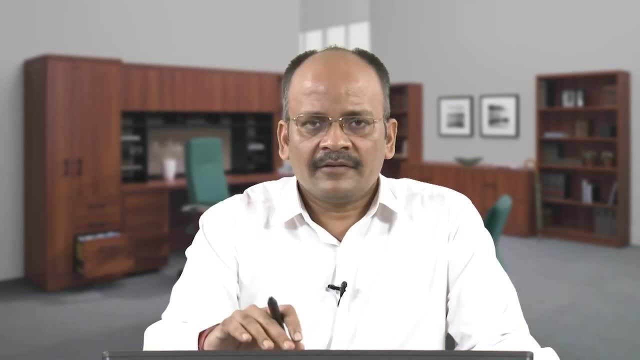 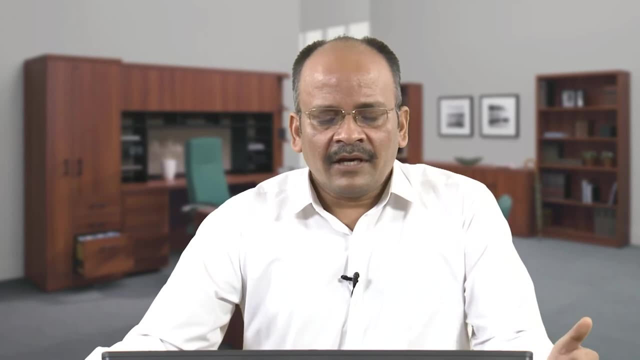 standard which have been decided by the central pollution control board. So this is very essential. Now the water collection system. starting with the first step is the wastewater collection system or water collection system. So what do they do So the water collection system actually transports the wastewater from its origin? may be industry. 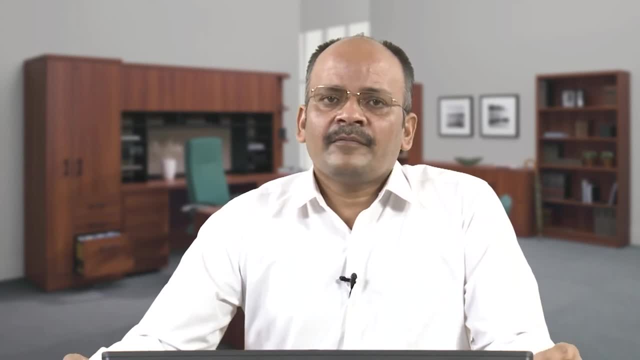 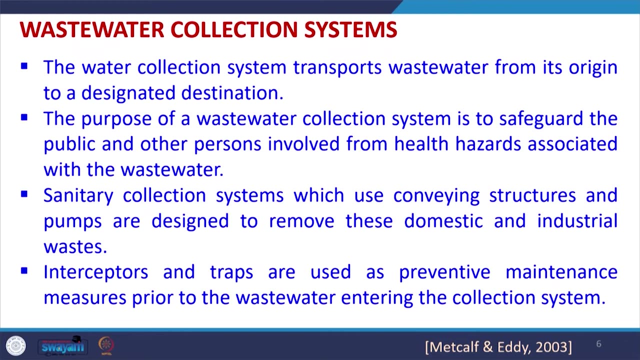 or manufacturing different residences where the water is being discharged to its designated destination, and that destination may be a effluent treatment plant, a common effluent treatment plant, a sewage treatment plant, etc. So depending upon that, that destination may also vary and we have to transport that water. The purpose of wastewater collection is to 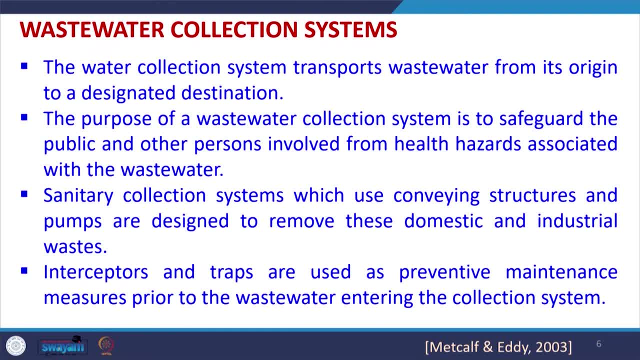 safeguard the public and other persons involved from health hazards associated with the wastewater. So we do not want water to be discharged from each and every home into the open channels because it will create unhygienic conditions, So a lot of sanitary issues and other things may happen. So this is very important. So sanitary collection systems. 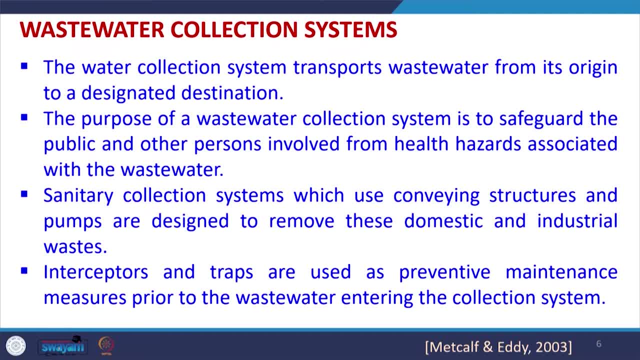 which use conveying structures and pumps, are designed to take these domestic and industrial wastewaters from their home. So this is a very important point. So the wastewater collection system is designed to take these domestic and industrial wastewaters from their discharge point to the designated positions and in between there are interceptors. and traps which are used for preventive maintenance also and to measure anything, that nothing is being discharged out of the collection system. So we always have preventive maintenance and for that we have lot of interceptors and traps which are being used. So wastewater collection system is. 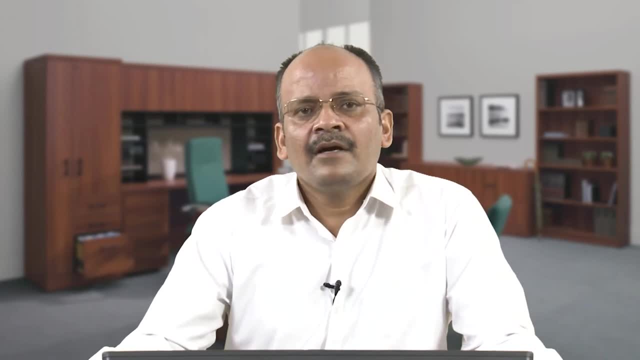 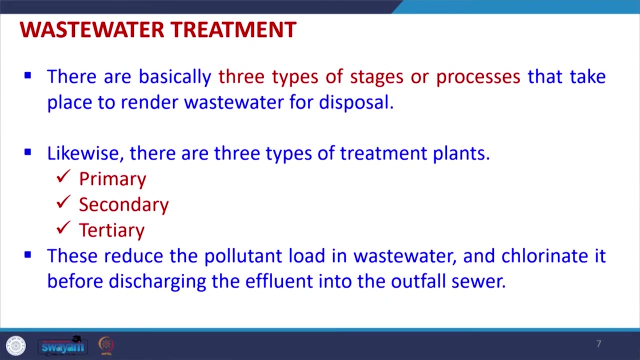 a different topic which can be discussed in length Now further. after collecting and transporting it to the treatment plant. So treatment plant where wastewater is further treated. Now there are lots and lots of possibilities of different units and how the water is being. 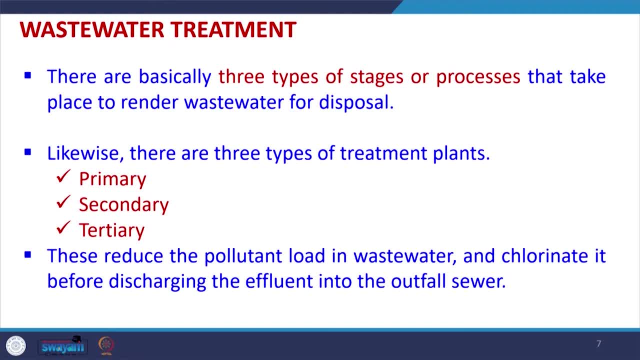 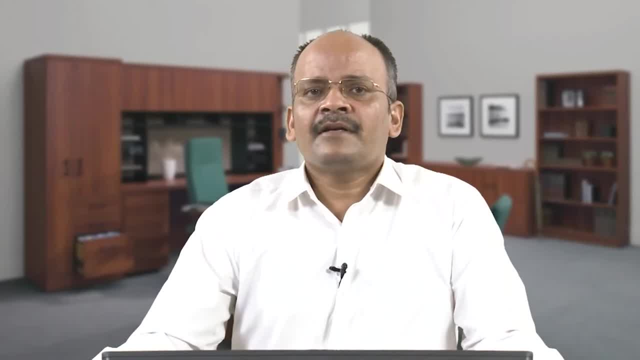 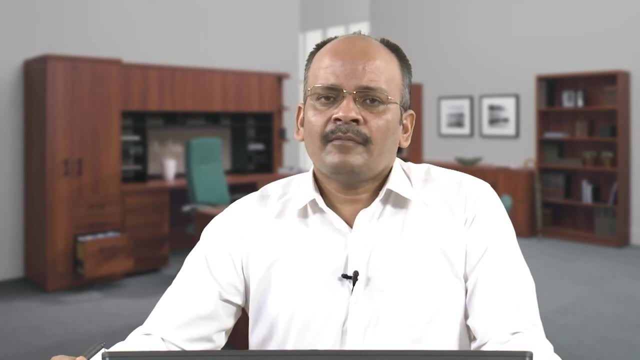 treated. So that will depend upon the characteristics of water, amount of water being generated and what is the use. So all the 3 things decide that which type of units are to be used in the treatment plant. So if the water is to be used for drinking purpose, the treatment strategy will be: 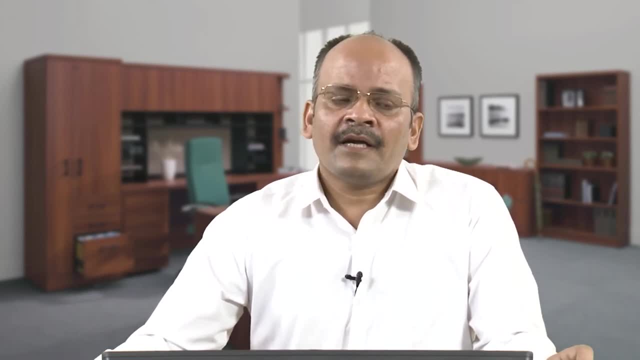 different Within drinking purpose. suppose water is being collected from river, So its characteristics will be different, So treatment strategy will be different. If water is being collected from a lake or reservoir, or water is being taken from the ground, then the treatment strategy will be different, though the designated use is same. 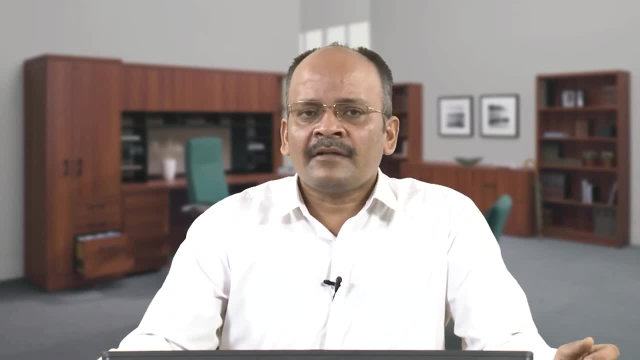 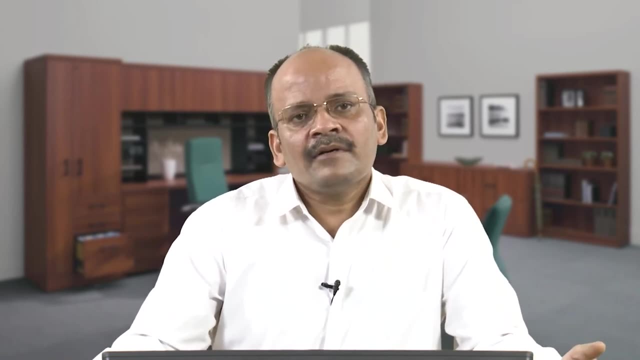 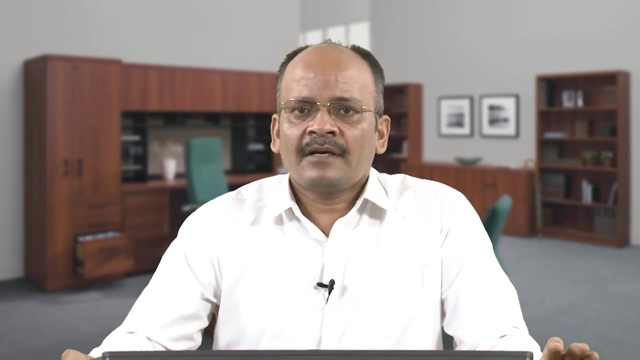 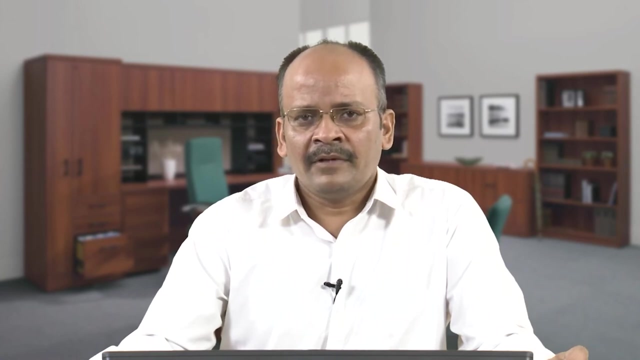 that is for drinking. Similarly, if the water is coming out after its uses from the industry or from the residences, then treatment also will be different. But broadly we can classify overall treatment processes as three types of stages or processes that take place whenever we have a water treatment plant or wastewater treatment plant. It is possible that- and these stages or processes are broadly called as primary treatment, secondary treatment and tertiary treatment- There is a pre-treatment also, pre-primary treatment also, and there is a high possibility that in one of the units, depending upon 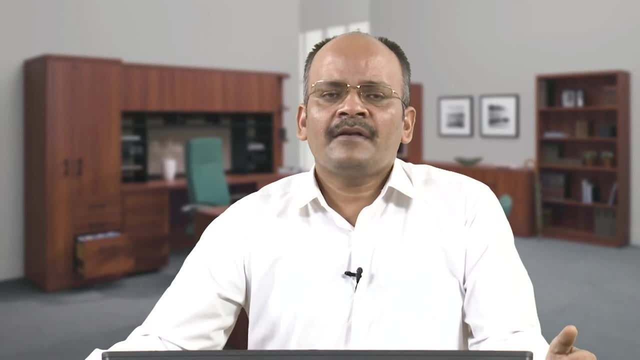 upon the requirement and from where water is being taken, being treated. So there may be only primary treatment may be there only. there may be place only primary and tertiary treatment is only there. there may be place where primary and secondary treatment is only there. 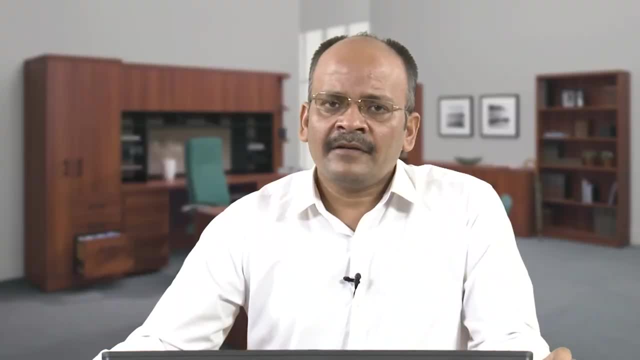 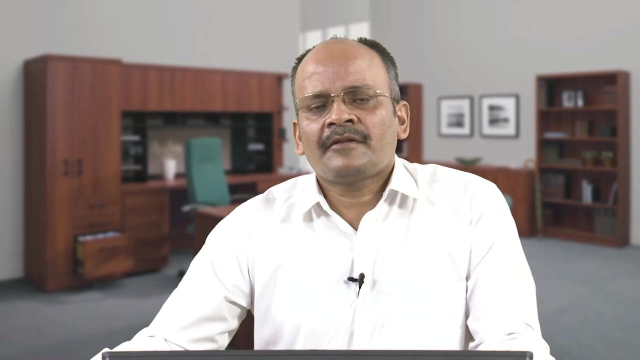 So it depends upon the various factors that how we decide which units have to be used for treatment, but broadly we can classify them as primary, secondary and tertiary, and we are going to learn little bit about primary, secondary and tertiary treatment in the next. 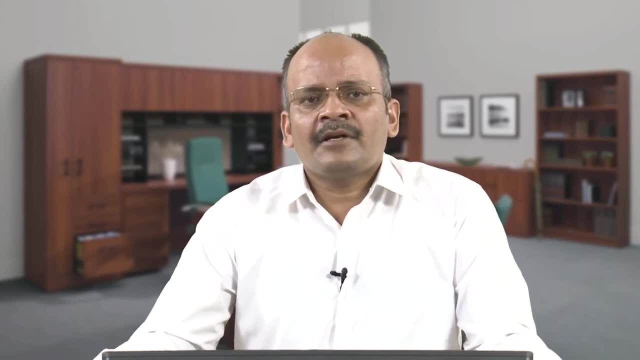 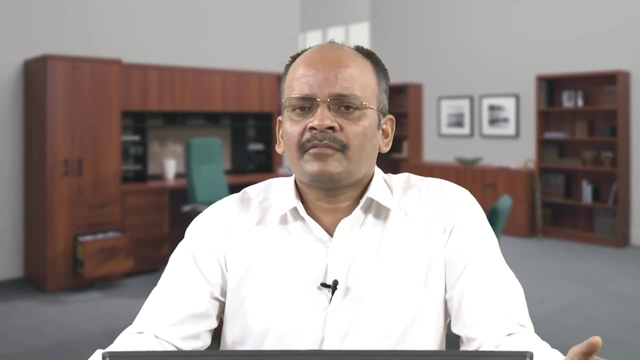 few slides And these treatment. actually they reduce the pollution load in the wastewater. and for suppose we have to use the water for drinking. So sometimes chlorination has to be done before using it for potable. Similarly for effluents also, there is a possibility that this is not possible. 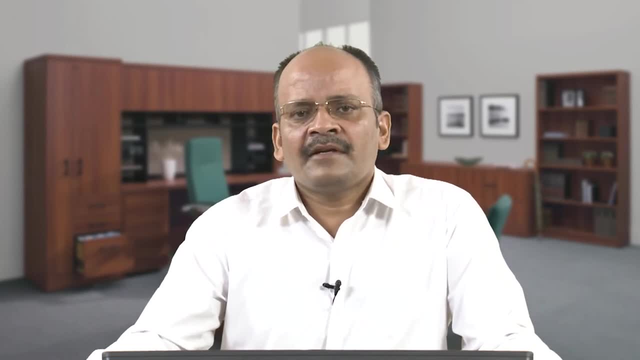 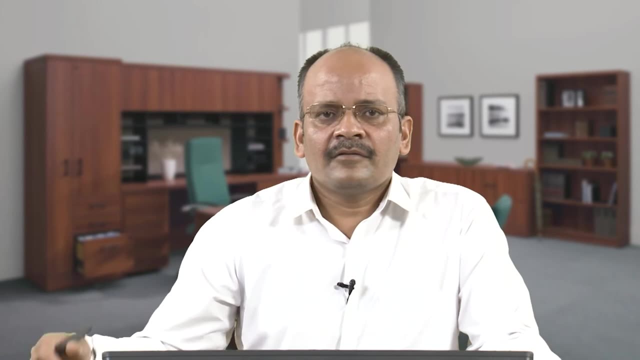 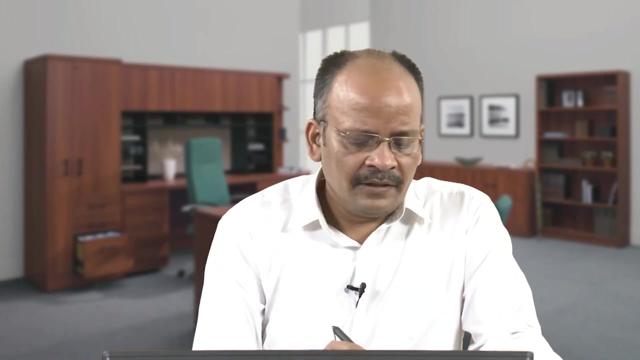 So disinfection or chlorination is done before discharging the effluent into outfall siever or any other place where it is being discharged. So this is there. So we will try to understand each of the primary, secondary and tertiary treatment. 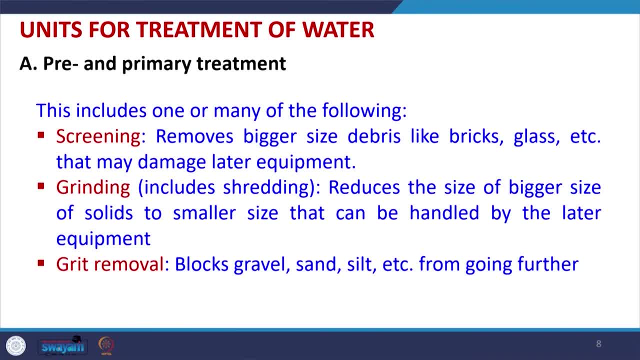 in little bit detail now so that we can further understand what are these processes and how they are used in the So, starting with pre or post So pre and primary treatment. so they have few objectives. they are broadly used for removing bigger size particles out of the water and also inert materials and other things. 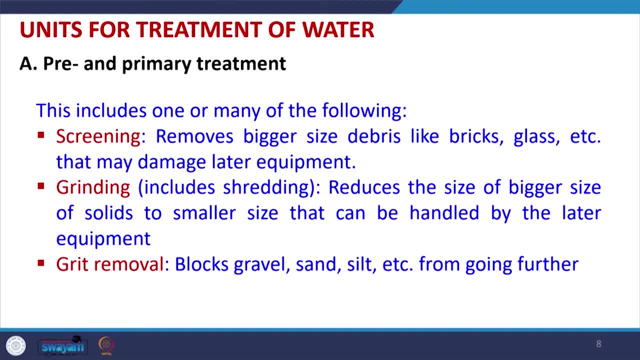 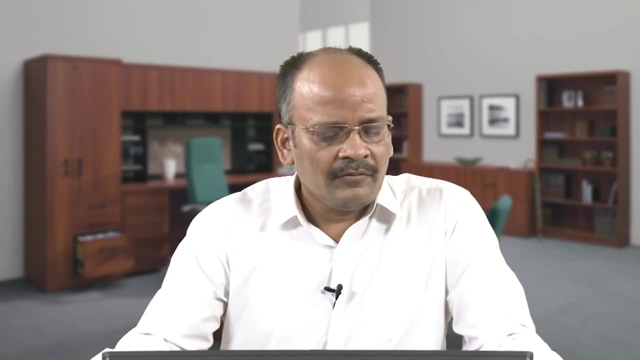 So their purpose is to treat the water in a very simple manner and generally physical treatment is more there as compared to other treatment like biological, physical and chemical treatment is general. So these include, may include, one or all of the following which are discussed now: 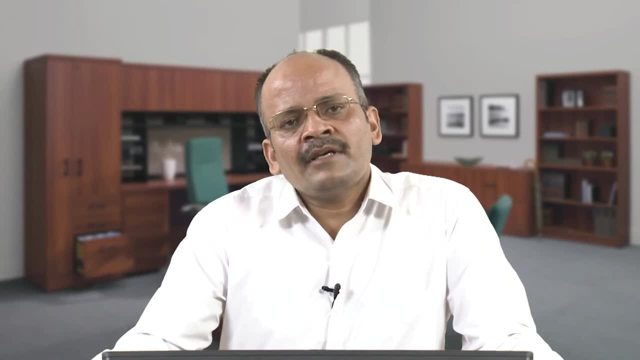 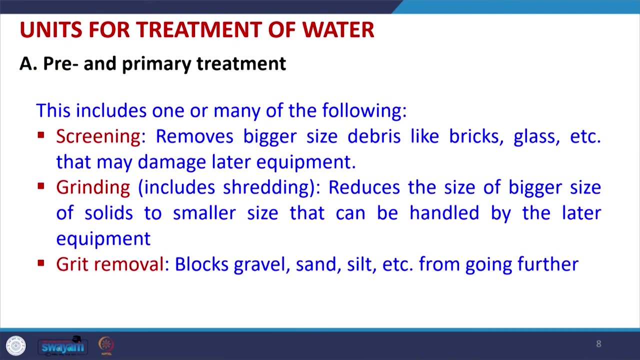 So screening is the first step. So in the screening what we do is that we remove bigger size debris like bricks, glass, etcetera and that may damage later equipments. So what we do is that we try to remove all these things during the screening stage. 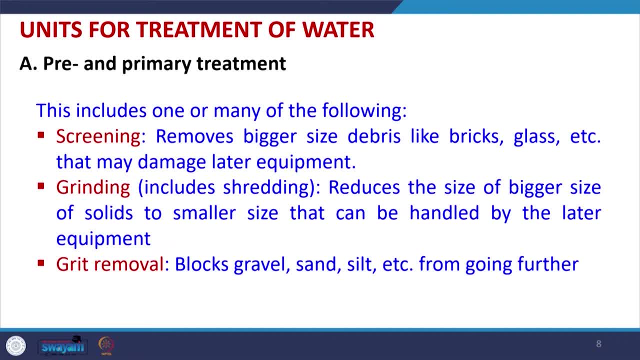 Similarly grinding or shredding. in this, what we do is that, after removing all the inert materials like bricks, glass, etcetera, whatever other solids maybe present- So they are further shredded into a smaller size so that they can be used, or they can. 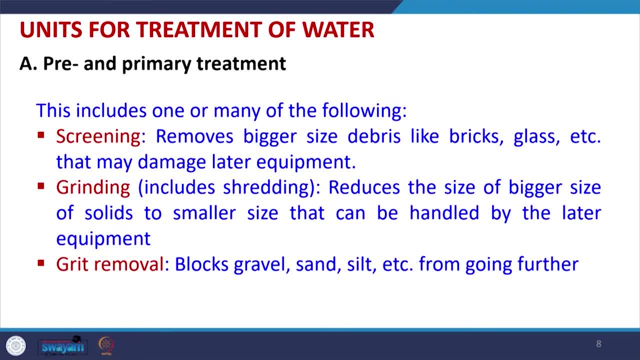 be handled by later equipments. We do not reduce the already smaller size particle. we only reduce the bigger size particles into smaller particles so that we can remove. So it is possible that this unit may not be there. it is also possible. 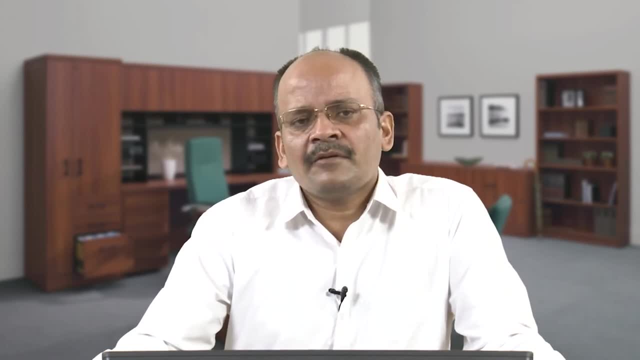 So depending upon the characteristics of water, this unit may or may not be there. Then in the grit removal we block all the gravel, sand, silt, etcetera for going further because they have only to be filtered out or removed. We cannot. there is no further treatment. as such, they are not changed into any other form. 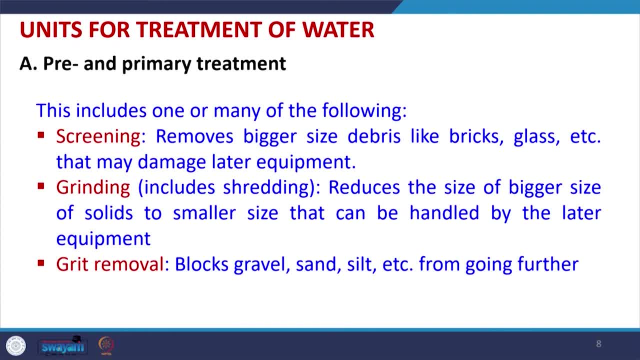 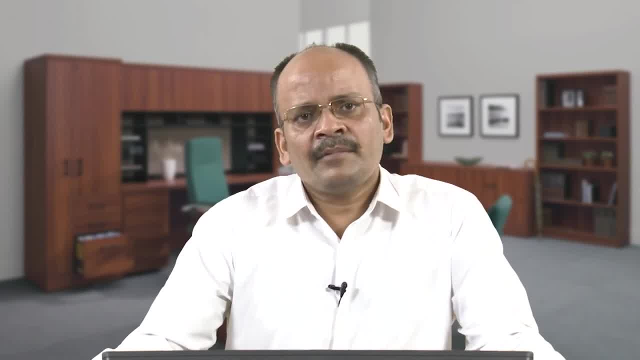 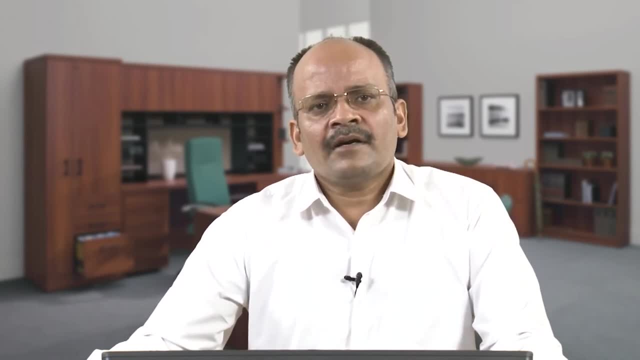 during the treatment. So it is better to block them or filter them out beforehand. so it is like called as grit removal. Now there is a flow equalization basin which is there in the primary treatment and it helps in equalizing the hydraulic or organic loadings to a certain optimum value for maximizing. 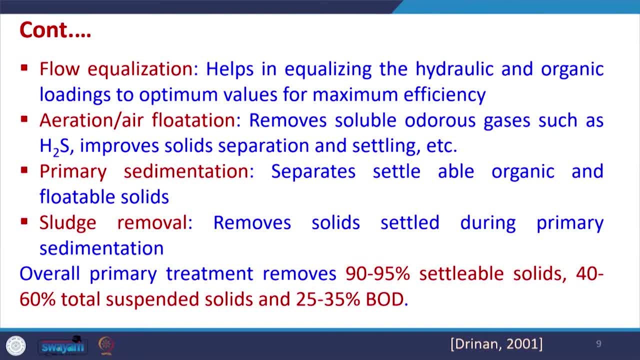 the efficiency of treatment. So this flow equalization, we will understand it helps in many ways And actually it equalizes or homogenizes the all the hydraulic and organic loadings. So that means we can use the treatment plant always at a optimum condition. 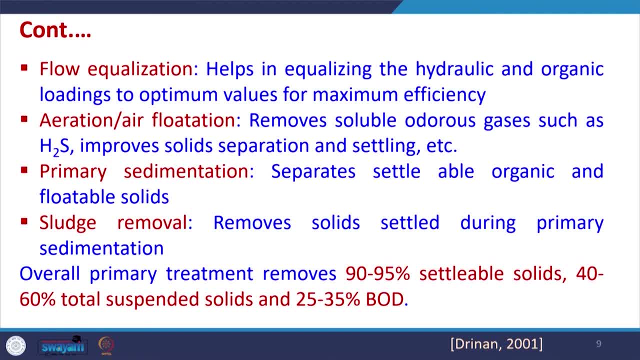 So it actually maximizes the efficiency. we will discuss each of these things in detail: flow equalization, aeration, primary sedimentation, sludge removal- everything we will be discussing in detail in 3-4 seconds, Thank you. So we have 3-4 slides after the present lecture, so we will be discussing each of the things. 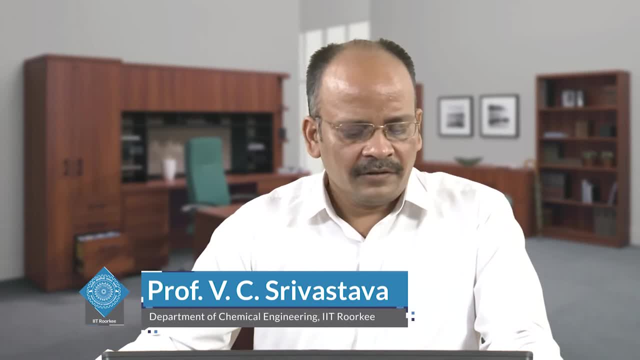 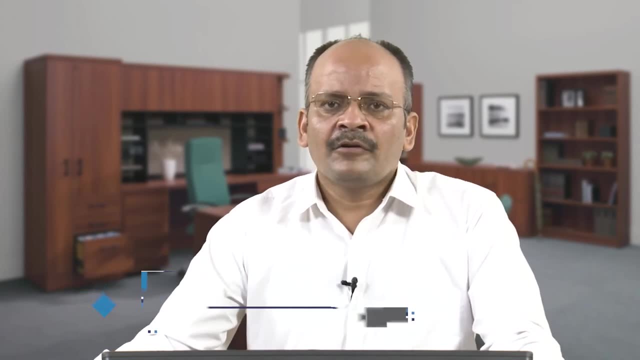 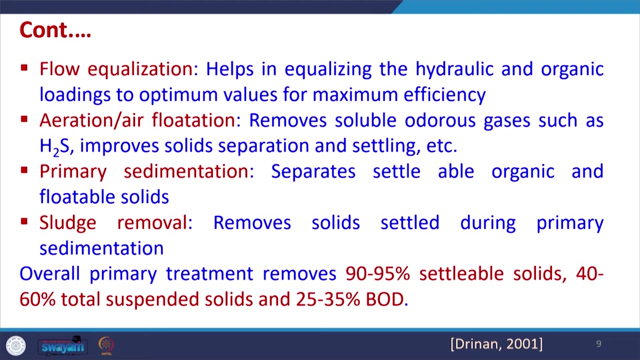 in very, very detail, solve some problems, etcetera- also for each of the units. Then we have aeration or air flotation unit, so their purpose is to remove any odorous gases such as H2S, etcetera, present: remove, improve, solid separation and settling also. 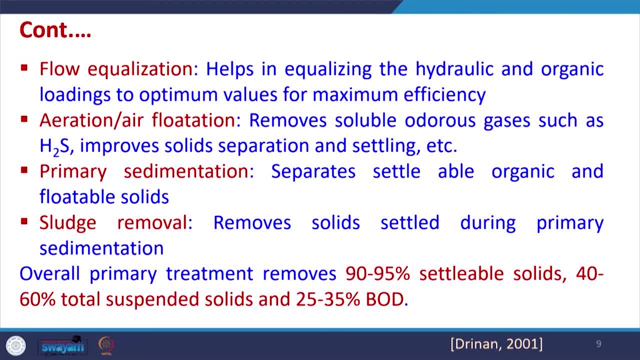 remove. like iron and manganese, Their removal is also possible. So there are multiple uses of aeration and flotation unit. It is also possible that flow equalization and aeration unit may be together also ok, So it depends. we can use them in together also and we it is possible that one of the 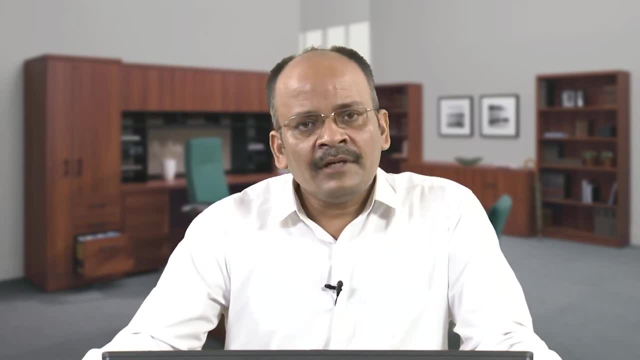 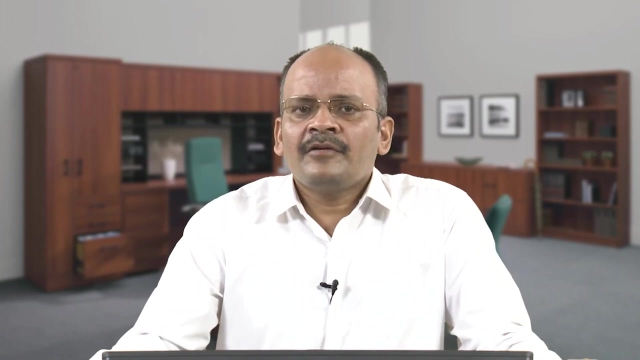 units may not be there. also, After that we have primary sedimentation. So what we do is that We try to settle out maximum amounts, So amount of organic and floatable solid or settleable solid, during the primary sedimentation. So during this process we may use some coagulants, flocculants, etcetera for removal of these. 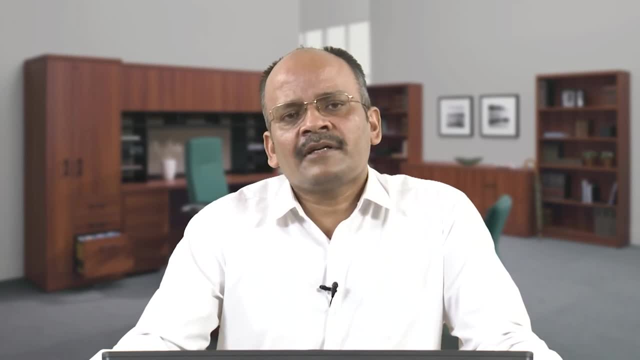 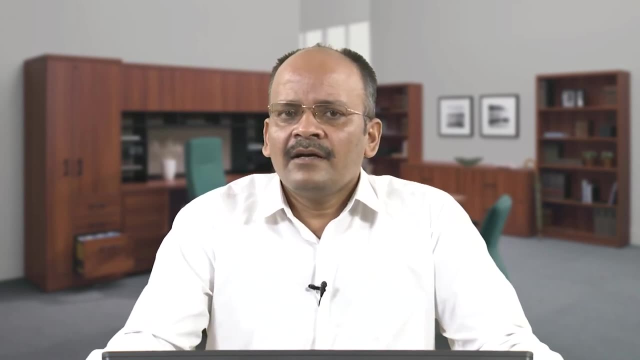 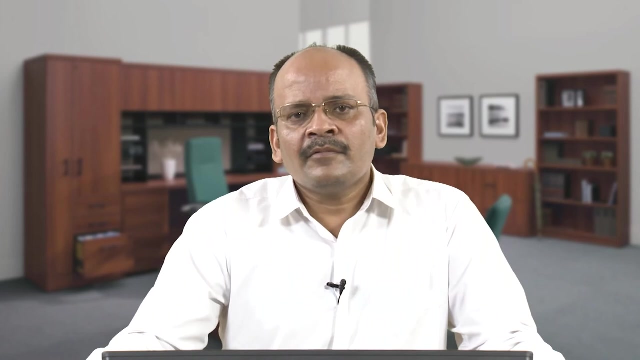 and we may use some filtration units also, as in the grit removal, for further removing some of the primary bigger solids, etcetera. In the sludge removal, the settling that happens of the after primary sedimentation, we remove the solid, try to settle them out so that we can further treat them later on. but- and the 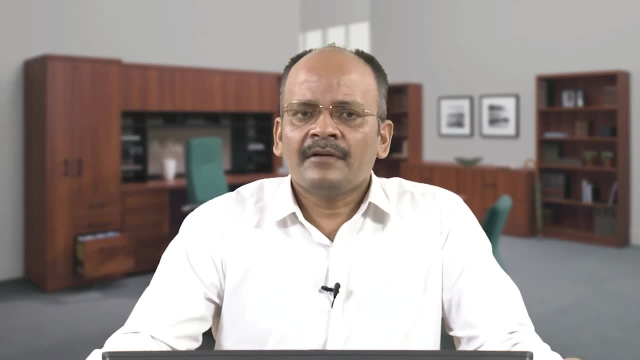 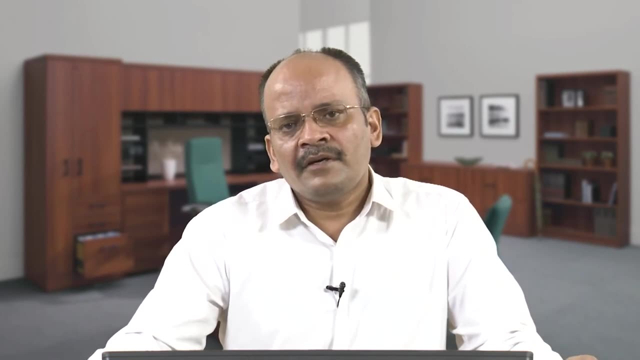 water after the primary treatment. generally it removes. it has already 90 to 95 percent of the settleable solids already removed. So this is the good thing that we can remove lot of settleable solids- Settleable solids beforehand. in the primary treatment itself then 40 to 60 percent of 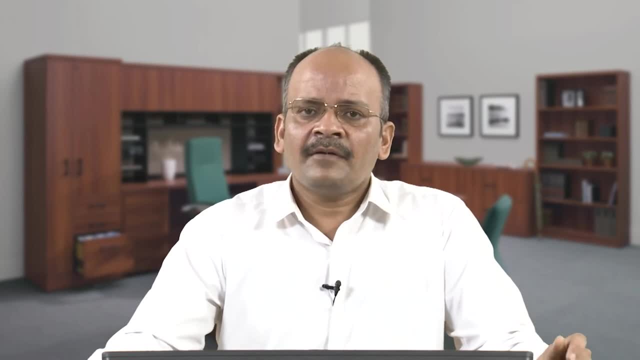 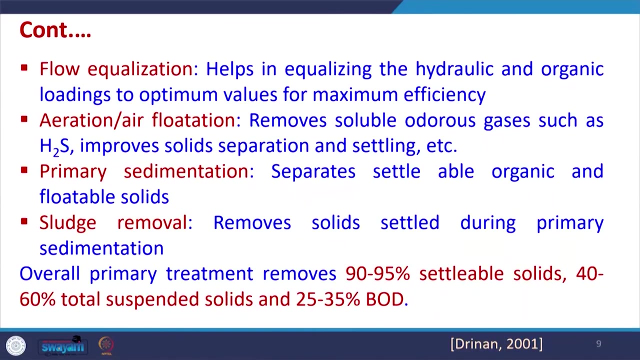 the suspended solids and 25 to 35 percent of the BOD load also. So if BOD load is getting removed, that means certain amount of COD load will also get removed during this overall treatment. So this is called primary treatment. it has some pretreatment units as well. 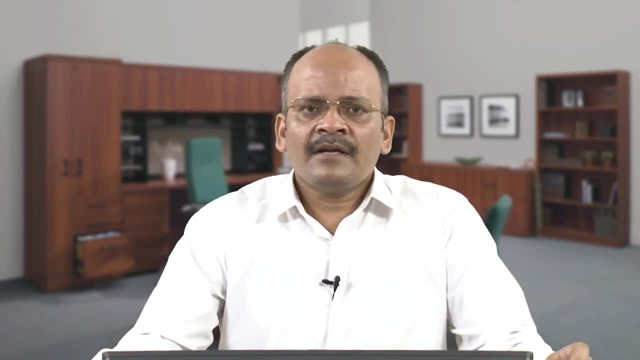 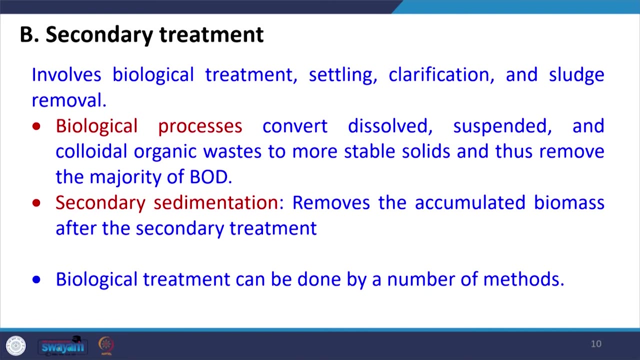 Then comes the secondary treatment. The secondary treatment is generally a biological treatment process, and in the biological treatment processes we use microoxidants which actually oxidize or degrade the organic matter present in the water after the one which is obtained from the primary treatment. So it is still, since we are only removing 20 to 35 percent of the BOD. so that means 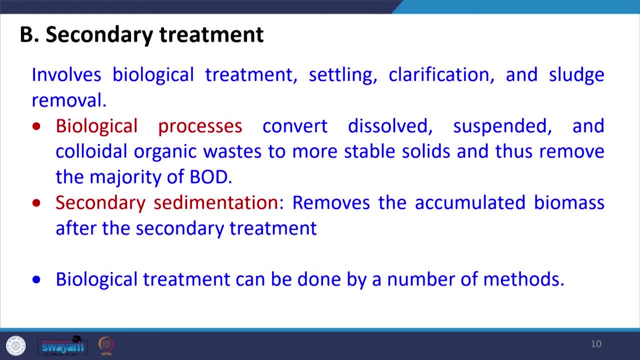 rest of the BOD has to be removed. So that means the rest of the BOD has to be removed, be removed here- and BOD means that we have to supply oxygen. So all the oxygen is supplied here, and microorganisms actually use the organics as their food material and they convert it into. 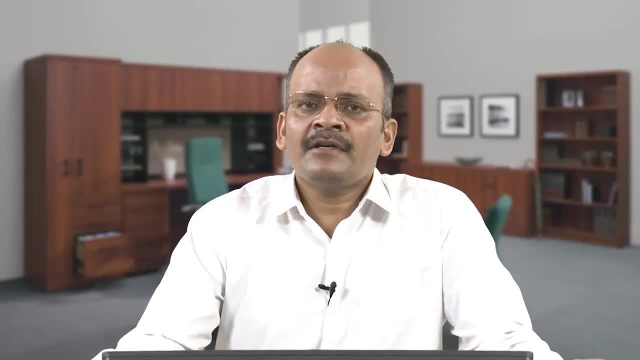 CO2, and during that process they may require oxygen, depending upon whether the process is aerobic or not. So in this case we have in the secondary treatment we have biological treatment. after treatment we settle out the microorganism and then we have clarification unit certainly. 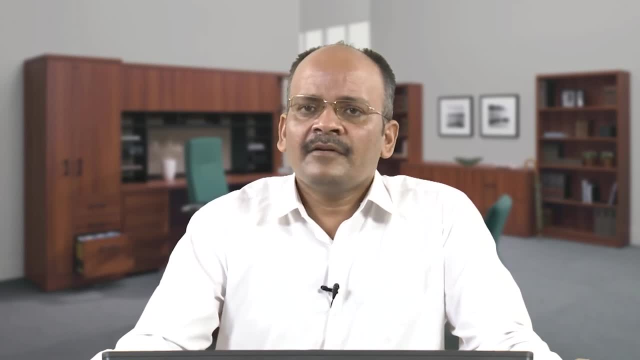 sludge is to be discharged, the solid waste, which will contain certainly some amount of water as well, it is a in the form of more, in the form of slurry, ok, thickened slurry. So this is there. So, and during biological process we convert the organic material, the dissolved, suspended, 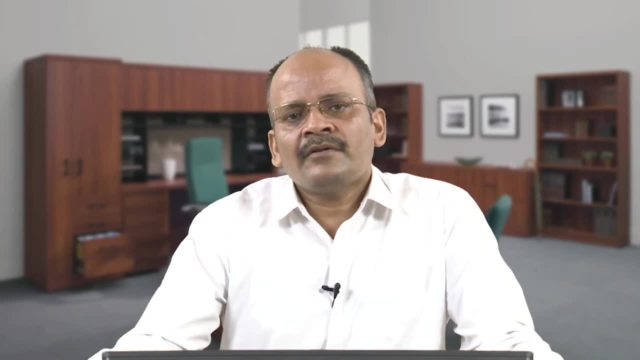 and colloidal organic waste into more organic material. So this is the way we do it. So we have more stable solids and during that process lot of oxidation happens, So CO2 may get generated if the process is anaerobic, So we have lot of gases which may also get. generated like methane, hydrogen, etcetera. So but majority of the places we have biological treatment in the secondary treatment is like biological treatment only. majority of the places it is aerobic treatment only. So some of the places is where the pollution load is very high and the BOD values and COD values are very high. Under those condition we perform anaerobic treatment also. It is done so that to convert the carbon into methane. So methane has lot of calorific value and we can use it for further for various purposes. So many a times the anaerobic 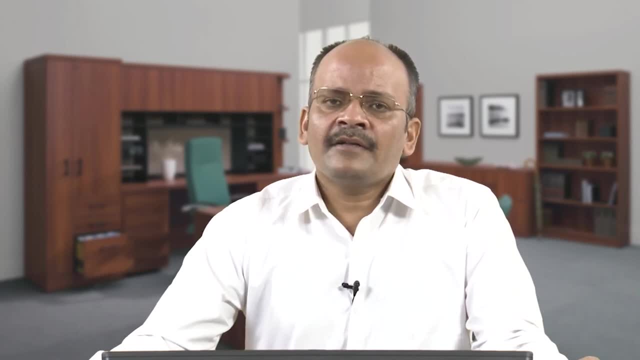 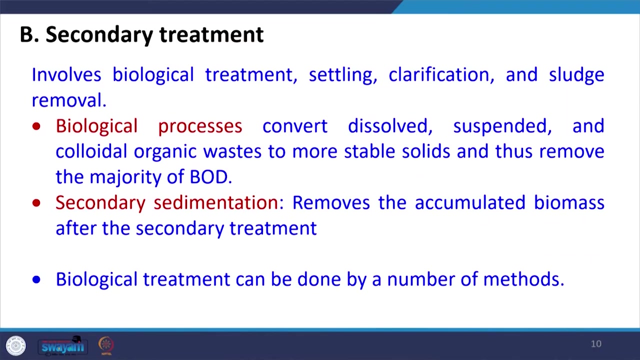 treatment is also possible in the secondary treatment, and it is done for those waste water which have very high carbon member content and high pollution load. So for them, after biological treatment, we have again a secondary sedimentation unit where the biomass or microorganism 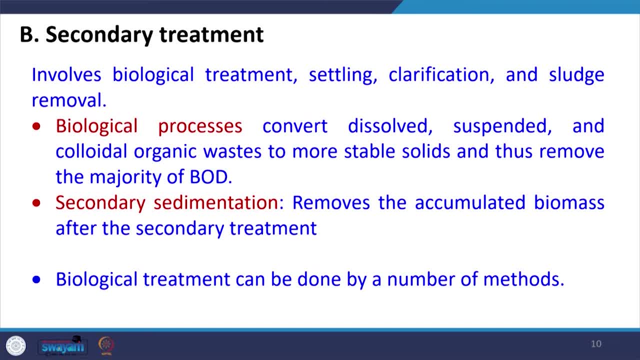 which have grown. they have to be removed because any of these units performed very well at certain optimum condition, And that optimum condition may be with respect to amount of microorganism present per liter. So it is done. So that is why we can do anaerobic. 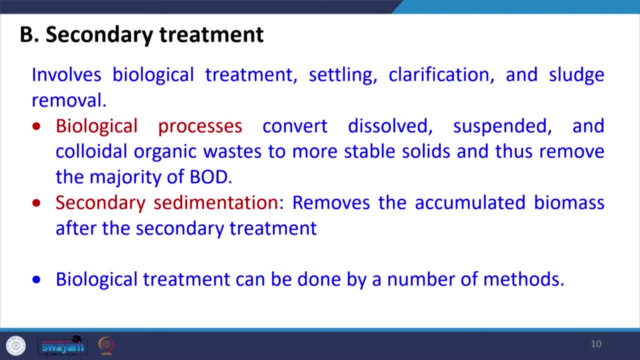 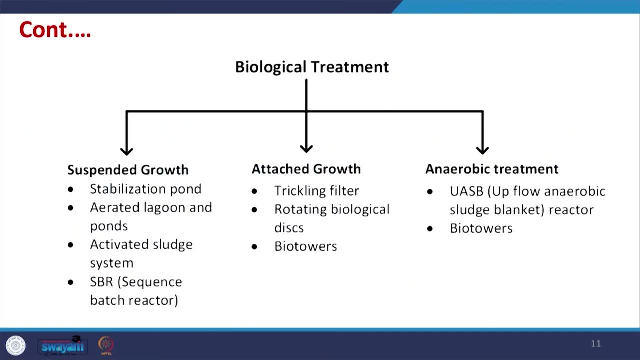 liter of the water being treated. So it is there. So biological treatment can be done by a number of methods which is described here. So we have suspend. three types of units are possible, So aerobic, anaerobic, this is broad classification. Then within these classification, we may have: 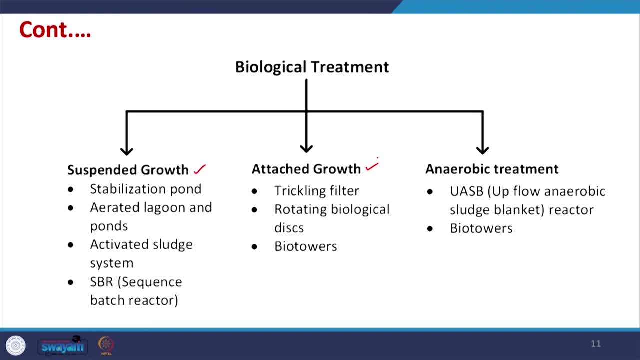 suspended growth. we have may attached growth also. So in the suspended growth we have stabilization pond, aerated lagoons and ponds, Then activated slush system, which is the most common unit in most of the treatment plant, Then SBR where sequential batch reactors may be there. 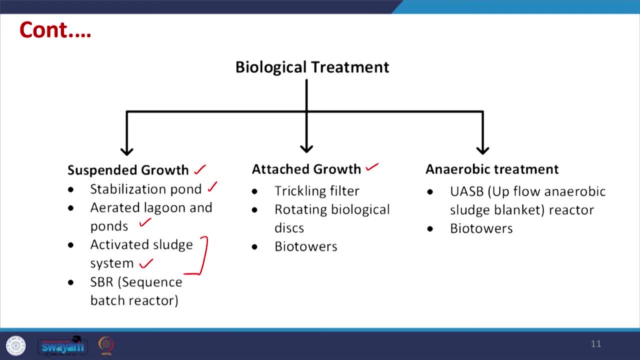 So that treatment is also possible. Attached growth systems involve, like trickling filter, rotating biological digs and bio-tivers, So this is also possible and all these are called attached growth system. Then we have anaerobic treatment on, among which USB reactor is most common, which is called as upflow anaerobic slush. 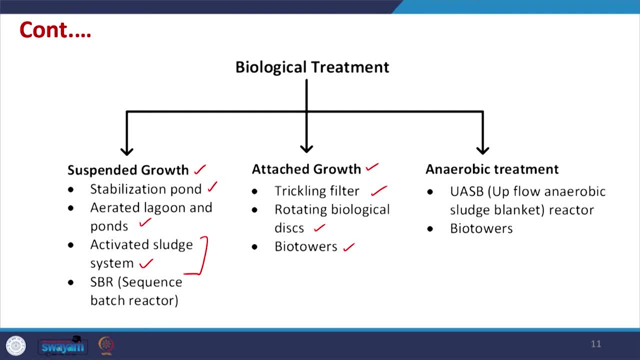 blanket reactor And in addition, the bio-tivers may be also be performing under anaerobic condition, So this is possible. So we have aerobic anaerobic treatment and there is a possibility of suspended growth, attached growth systems where micro-oxygen how they are there in the 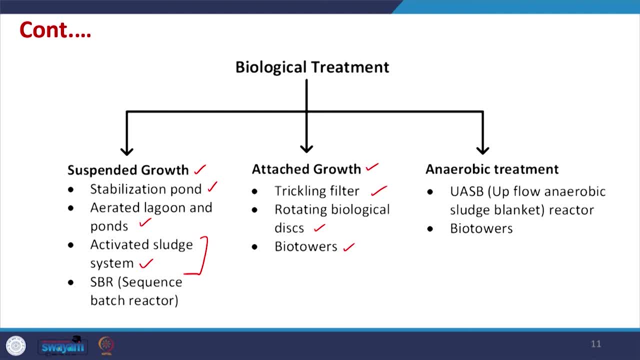 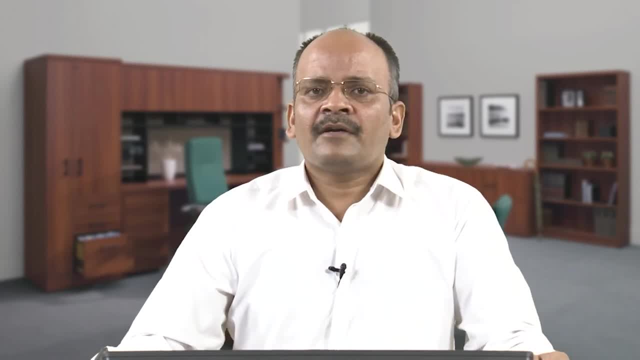 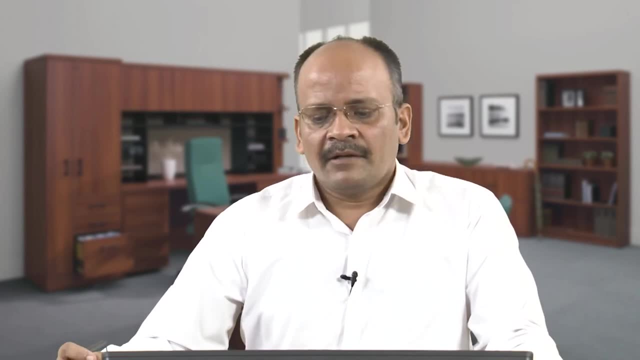 system. So, depending upon that, these suspended and attached growth systems are called as. So in this particular course we will not be learning much about biological treatment, because we have to learn only more about physicochemical treatment, not biological treatment, in this course. But you can still study them in detail. 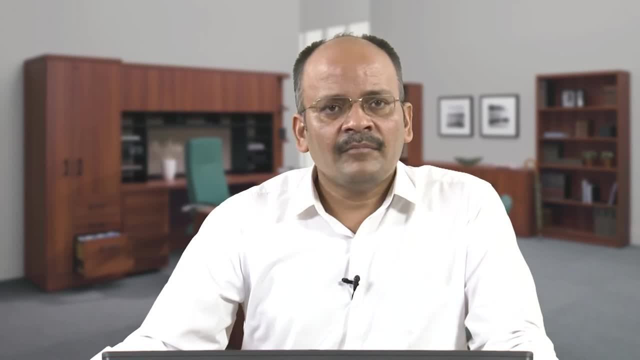 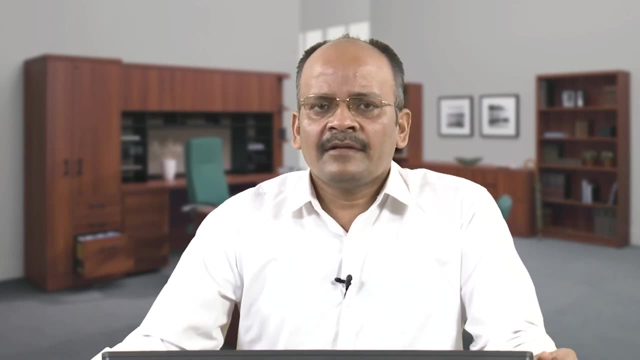 in other places. Then we have tertiary treatment. This may or may not be required, So depending upon the various end. So these are the uses. this may be there or may not be there, And so one of the most common things which are listed here they these are called tertiary treatment There. 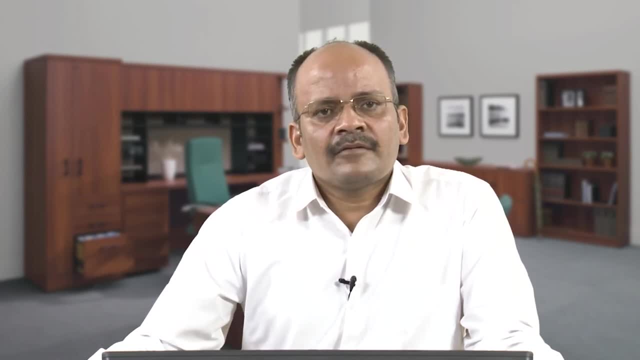 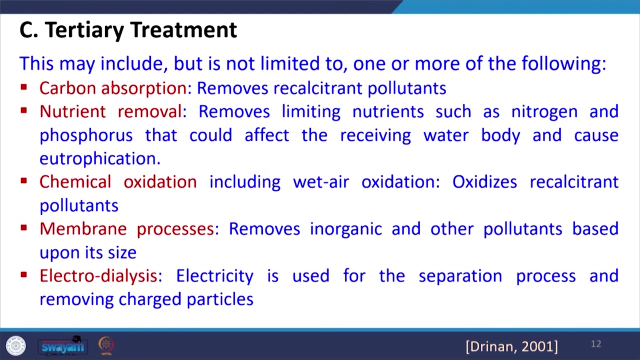 are many other techniques which are evolving And so these enormous research is being done in this area. So adsorption is one of them. absorption and adsorption, So they remove both, So this is more of adsorption, So this is possibility of a treatment adsorbing any recalcitrant. 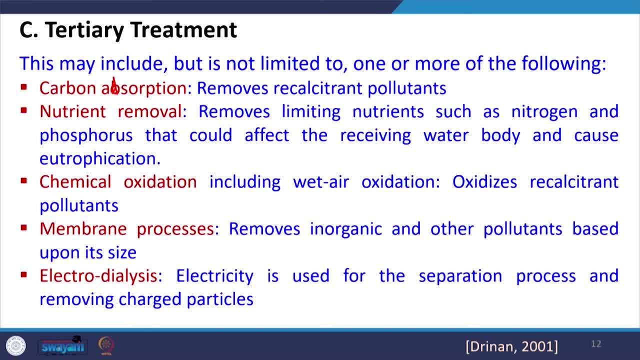 pollutant which is has not been removed. So there is a packed bed. In this packed bed we can remove the pollutant there itself. So will be studying in detail the adsorption process. Then we have nutrient removal. So earlier we had discussed that if any nitrogen and 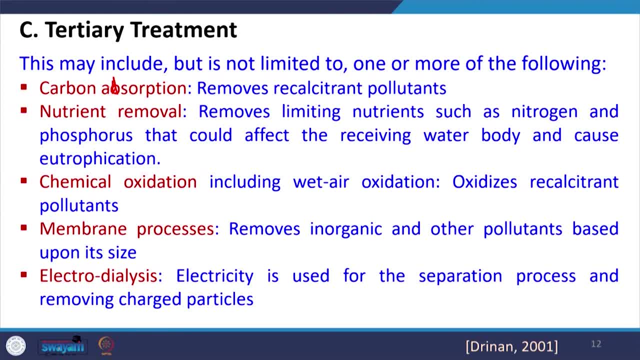 phosphorus. These are very important components. Then we have nutrient removal, So earlier These elements are present in the water and they are considered to be the essential elements for growth of any microorganism or aquatic plants or anything. So that means if we are discharging any water which contains nitrogen and phosphorus. so the receiving body will contain nutrients. So if nutrient, amount of nutrient in the receiving water body increases it may cause eutrophication, the growth of various water related plants, So slowly and slowly that lake or reservoir may die out because it will be totally covered. 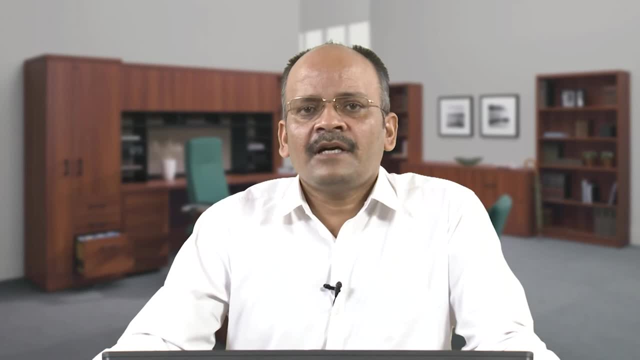 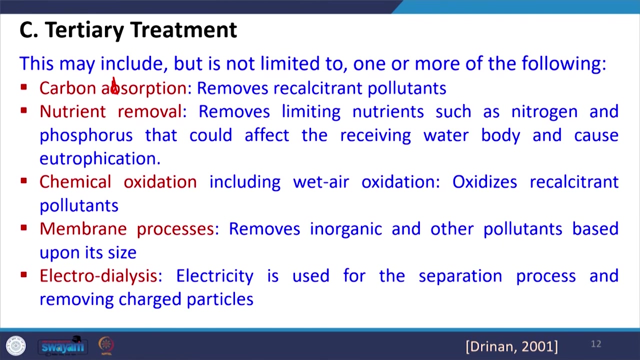 with the water plants, which is not desirable. So that is why it is very essential to remove the nitrogen and phosphorus beforehand. Similarly, there is a chemical oxidation process. Many times it is also referred to as, at many places, advanced oxidation processes also. 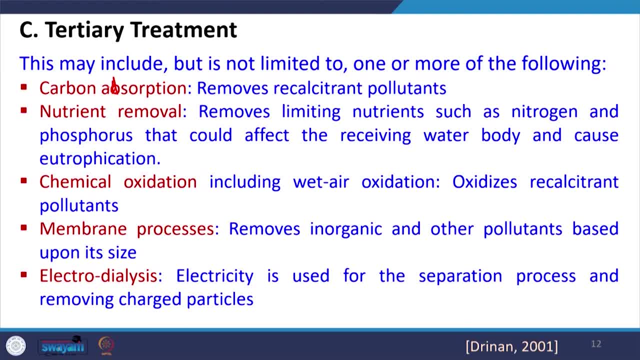 So again, So that means they oxidize any recalcitrant pollutant which is coming still present in the effluent discharge after secondary treatment. So, and this is possible if that chemical compound is highly like aromatic in nature. 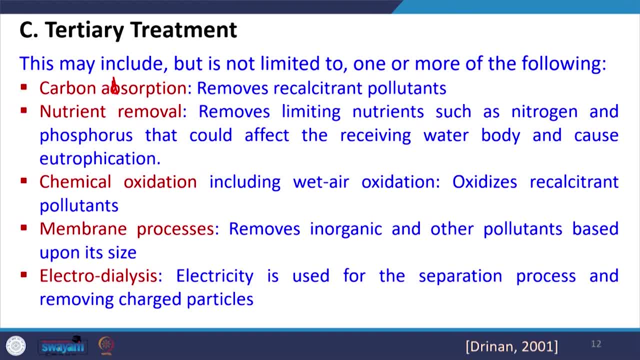 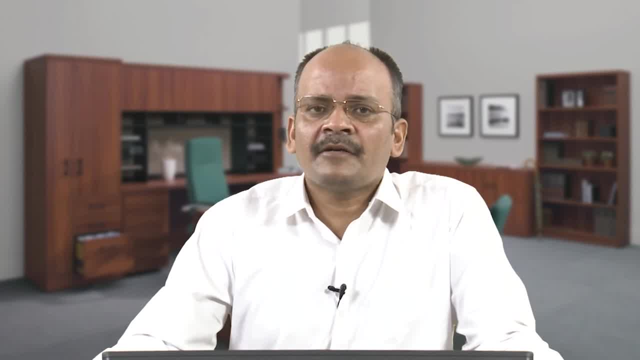 So it will not be broken down easily by microorganisms. So it is possible that that compound still be present after the primary secondary treatment. Also, for many wastewater, secondary treatment, So secondary treatment, is not possible because they contain so much toxicity that microorganisms 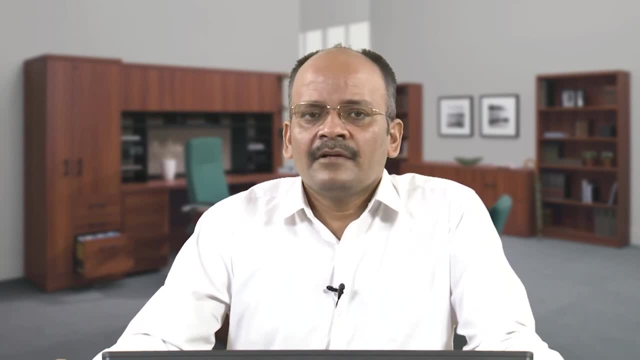 cannot survive in those toxic pollutants. So that is why we have to perform this chemical oxidation or advanced oxidation, and there are many techniques for this. We will discuss this in detail. We have membrane separation processes also, which involve, like reverse osmosis, ultrafiltration. 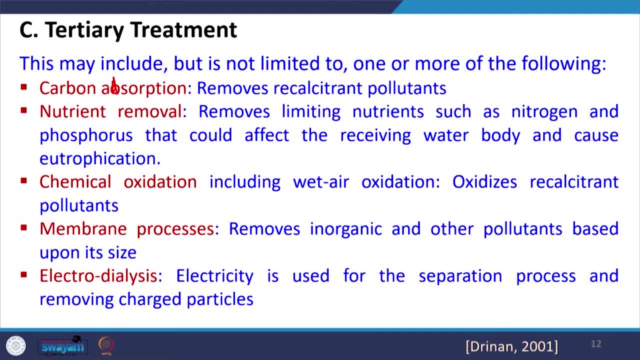 microfiltration And they remove various inorganic and other pollutants based upon their size. So the treatment strategy or membrane system that we use in the effluent treatment plant depends upon the characteristics and type of pollutant being present. So it is there. 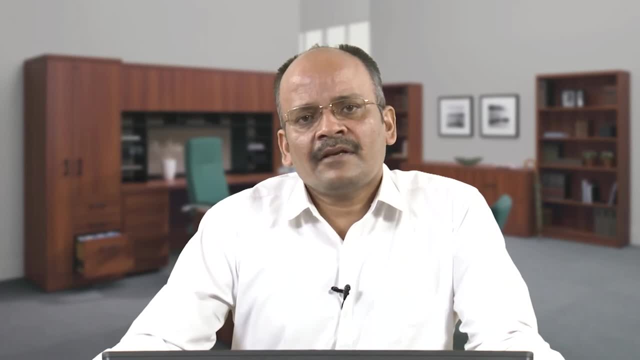 Then, similarly, electrodialysis is a technique which can be used for removing charged particles or ions. So now it is, It is becoming more common and lot of research is, etc. is being done for use of electrodialysis in various applications. 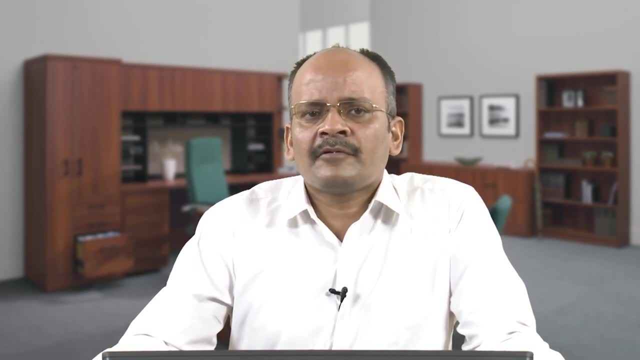 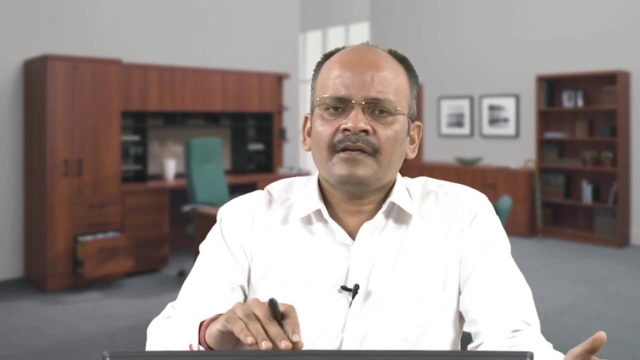 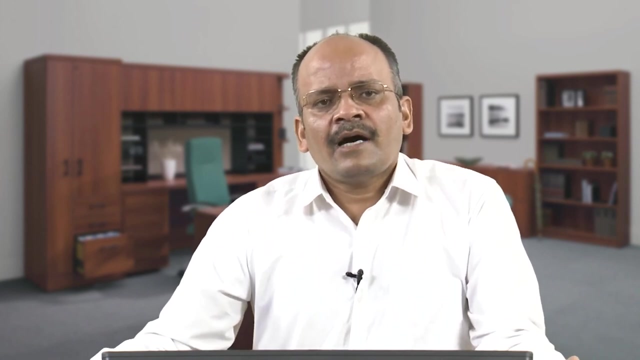 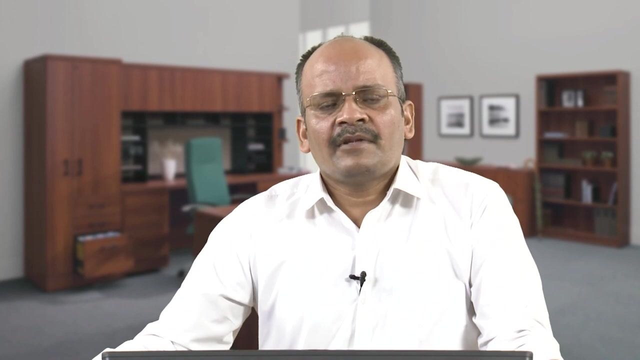 So there are similarly electrochemical treatment processes also which can be used for treatment of water in details, And these things, all these things we are going to discuss in detail and each of them will be discussing the basic mechanism, How they remove the pollutant, some basic idea regarding the design thing, and certainly 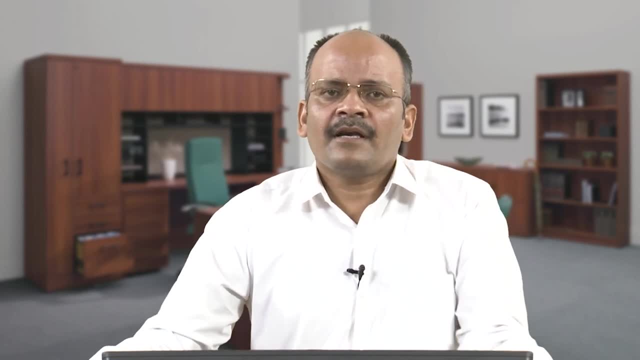 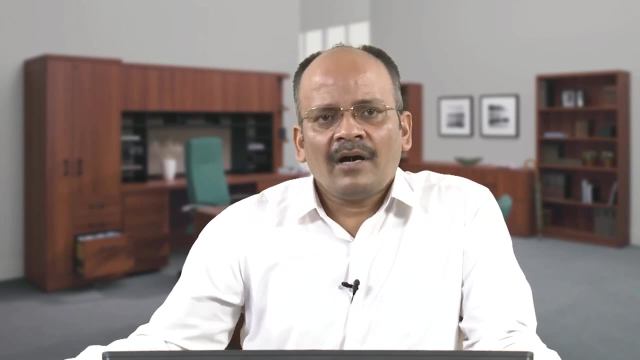 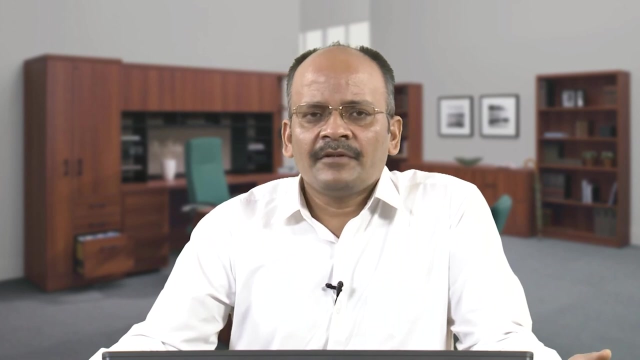 we will try to have some problems etc related to all these processes discussed in later sections of this present course. Then RO ion exchange: Ion exchange also removes lot of ionic pollutants by exchange processes and which is very common, in particular for removing the calcium and magnesium ions. 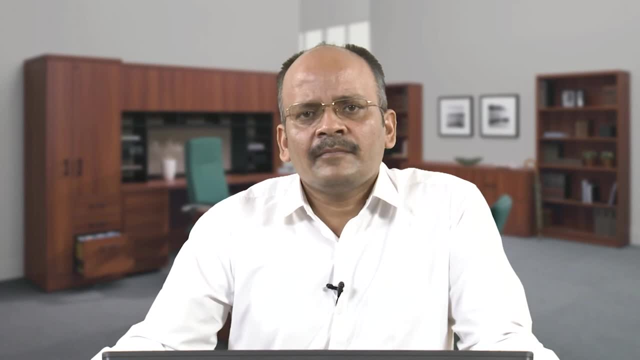 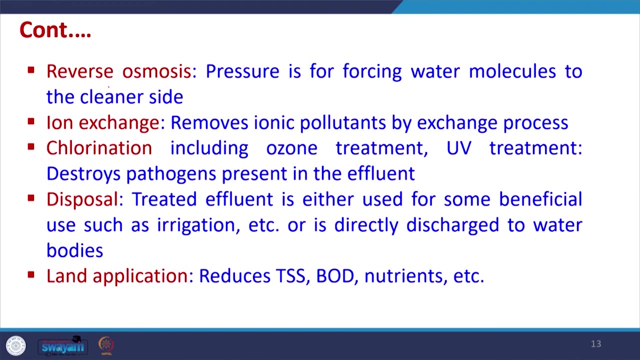 So this is very, very common. RO is also being used in many industries, etc. For actually they separate out the solids, So they have a concentrated slurry which is further evaporated in the evaporators, and we have a ZLD, which is there. 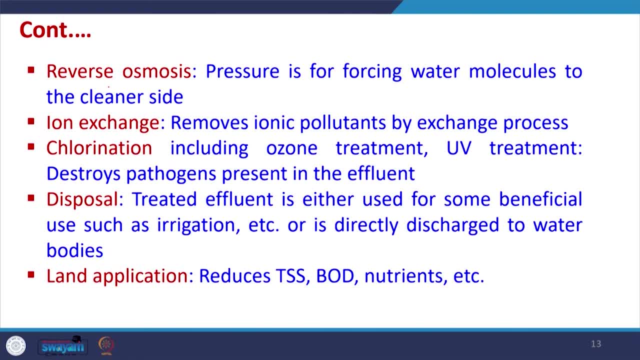 So they actually RO units. what they do is that if any water is coming which is having a certain concentration, So what they do is that they remove. So they remove the amount of very large amount of 80 to 90% of the water as clear. 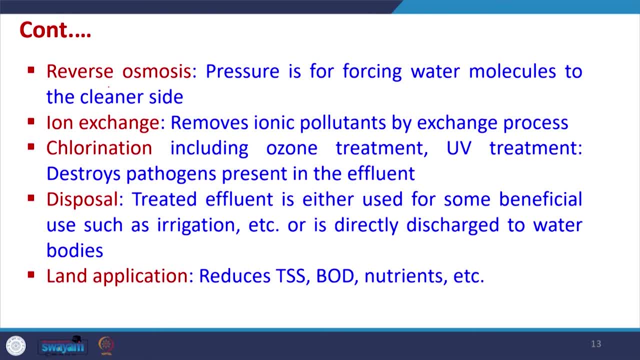 water and the slurry is further concentrated and that slurry can further be evaporated in the evaporators and we have a ZLD type of system. After certain treatments, after all these treatment, many times what we have to do is that We have to still destroy the pathogens. 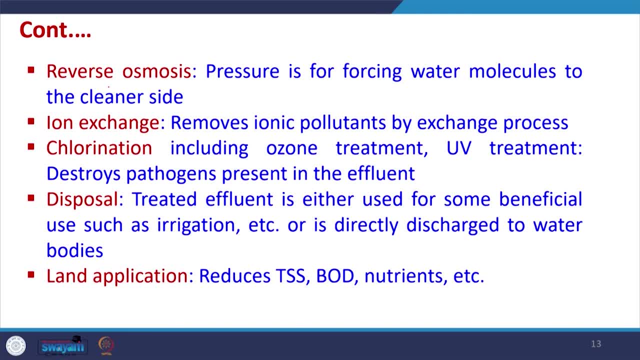 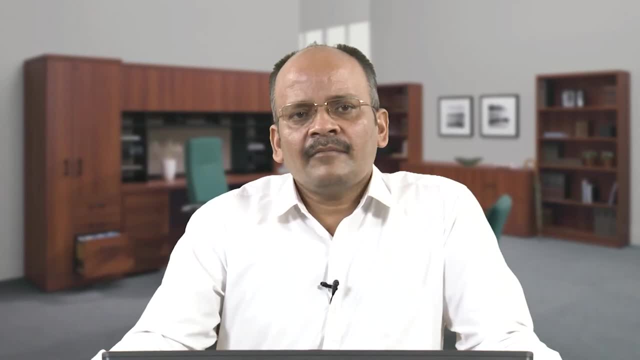 So that pathogens can be destroyed. So that pathogens can be destroyed Right including chlorination, ozone treatment, UV treatment, etcetera. So all these are possible for removing or destroying the pathogens in the effluent before discharge. And then finally, we have disposal. that treatment effluent is either used for some beneficial 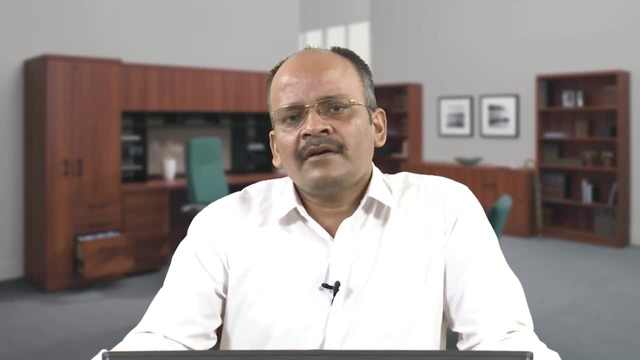 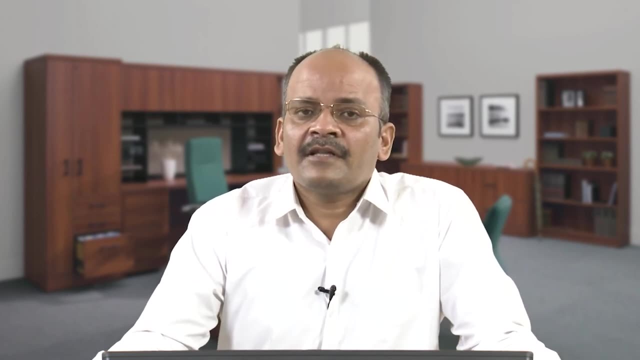 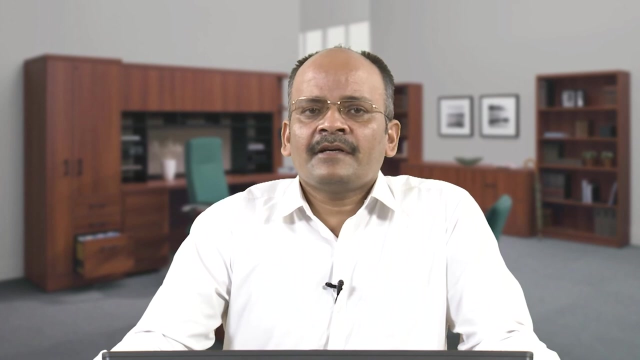 use within the like, irrigation, etcetera, or it may be directly discharged to the water body, or it may be taken to evaporator and further evaporated so that we have a ZLD system And also there may be a land application of the water also, So this is also possible. 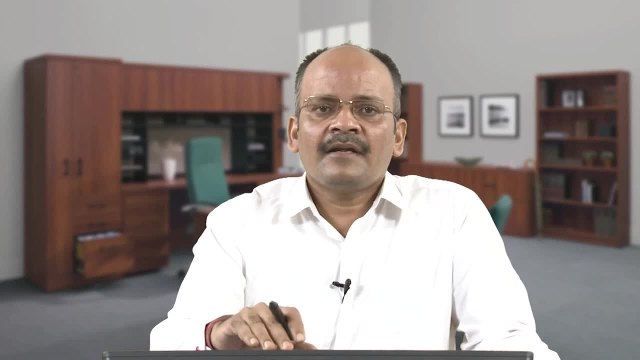 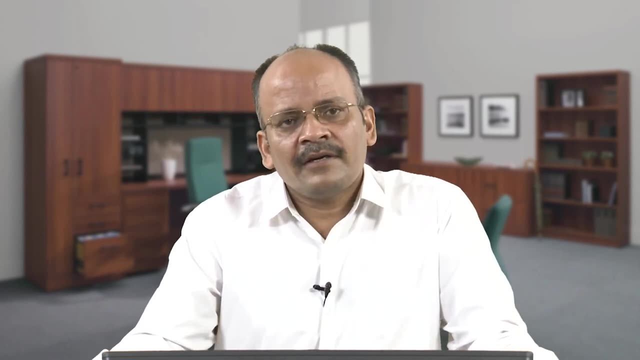 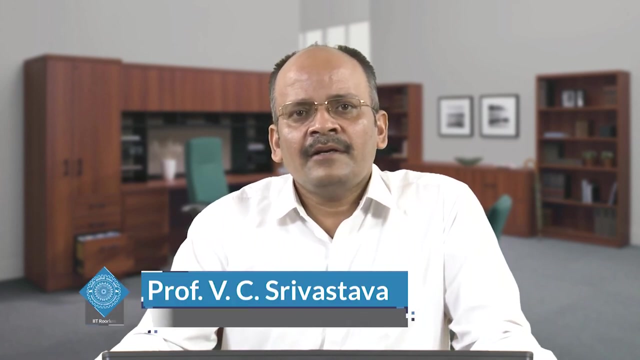 like in the case of sugar industry, the land application is possible. We have lot of solids. though they are do not form the part of biological, this overall treatment, but lot of solids come out And that solids have to be converted or they have to be. further treatment has to be done for overall management. 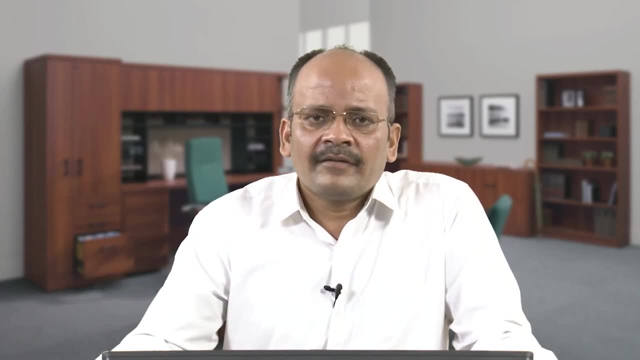 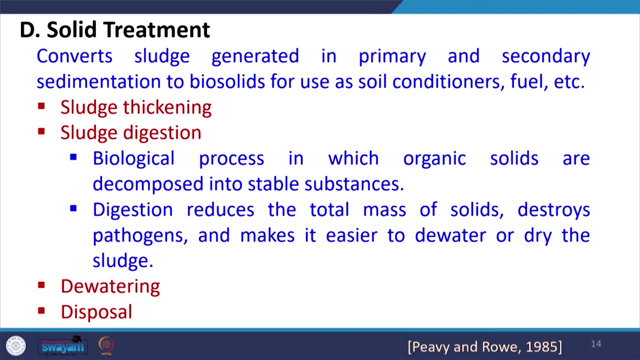 of the solid. So this involves sludge thickening, sludge digestion, So we call it as a sludge, So that sludge has to be thickened then digested. Digested means the organic solids are decomposed into stable substances and it may be anaerobic generally and it reduces the total mass of. 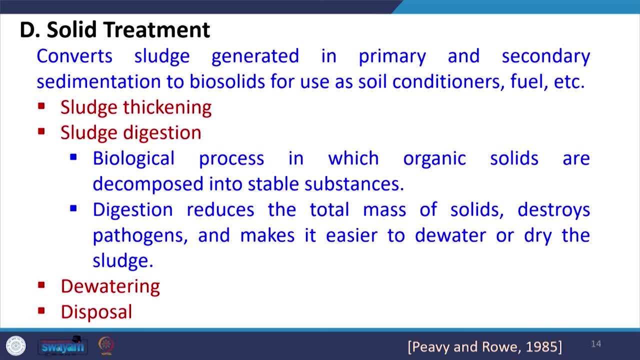 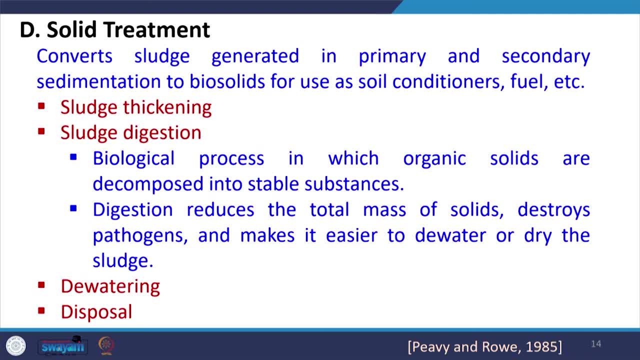 possible. So this is also possible. So this is also possible. So this is also possible- or for further use as a landfill, or maybe for getting energy out of that. So there are lots of possibilities of disposal of solids, depending upon the characteristics. 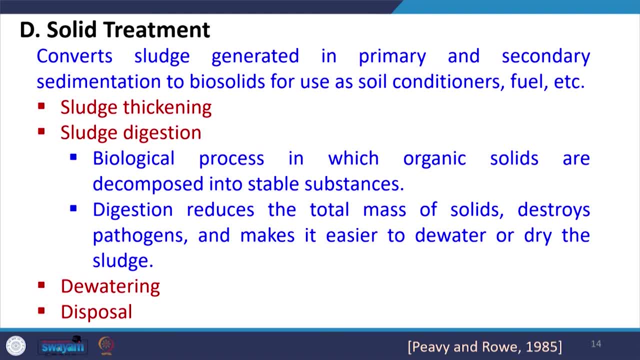 of the solid. So this is there. So we will discuss that in detail later on also. So this is how the treatment, overall treatment, works, and any of these units may be there, may not be there. This will depend upon the amount of water being generated, the characteristics of the.